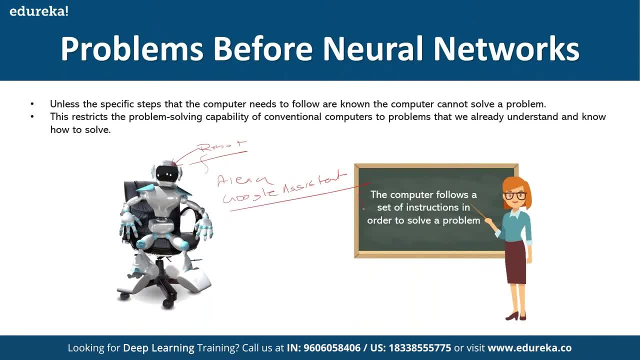 Okay, so these sets of instructions are required for the robot to take actions. Right, So these can be accomplished using neural networks. So, for example, once the robot decisions are made, know-how, that's what I'm actually generating. So now, how can you follow along? I am going to show you something, but right now I am not going to give you any ouija, Jim, like in your video class. I'm going to движ forward, because if you finally respond with qualifying in one word give or armрост in one parametric and month long, then a little白��. 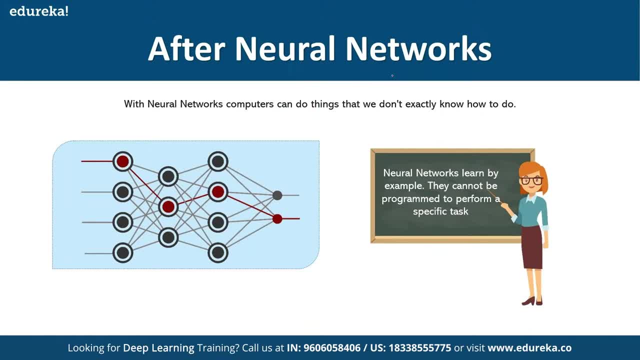 And the last thing that you need to do is 195 had not like an into timer. You just have to go to your internet list. this is how you know. we are going to develop neural networks and these neural networks are going to be trained. we are going to train it just like how human brains are trained. 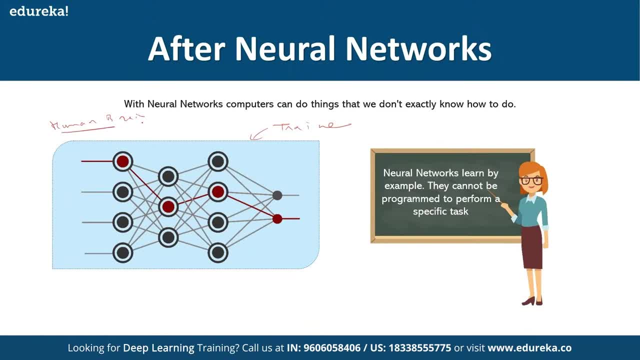 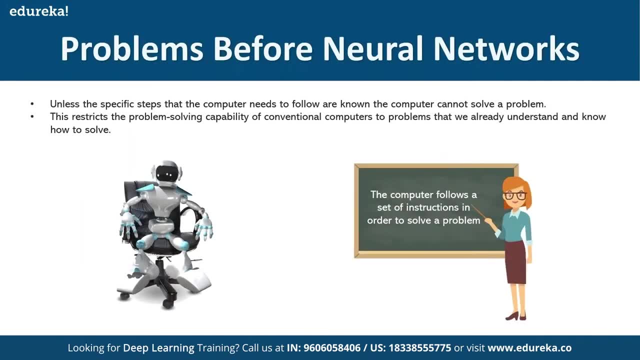 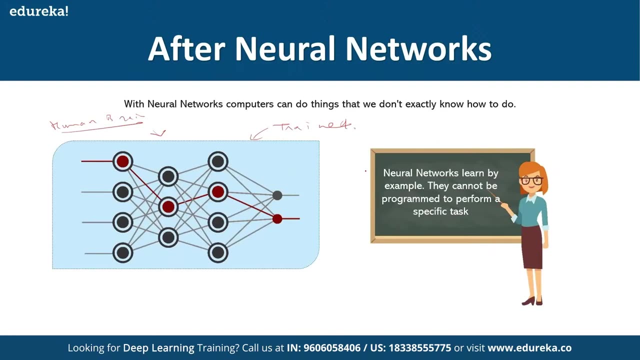 right, we are going to train something known as neural networks. post that this neural network will be deployed in the robot's mind and it will be able to follow some specific task. okay, how it is, what are neurons, what are neural network? we will understand in detail, but this is just the 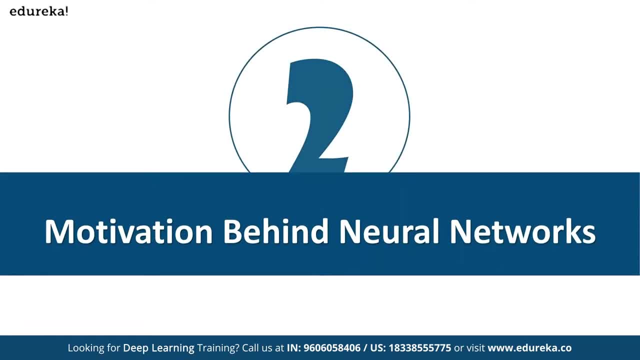 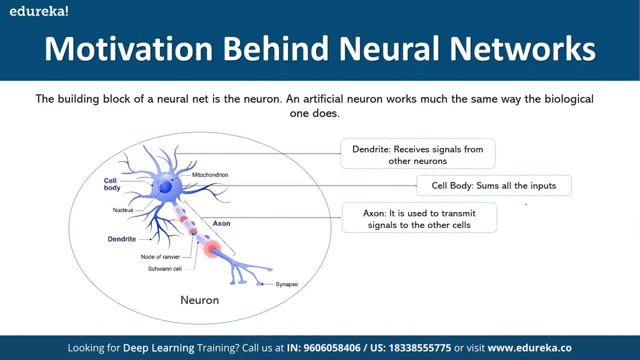 background of it. so what is the motivation behind neural networks? as I said, the human brain. so the building block of any human brain is a neuron. right, so it is neurons that is the building block of any human brain. so this is how a neuron looks like. so, if you see, it has a nucleus and 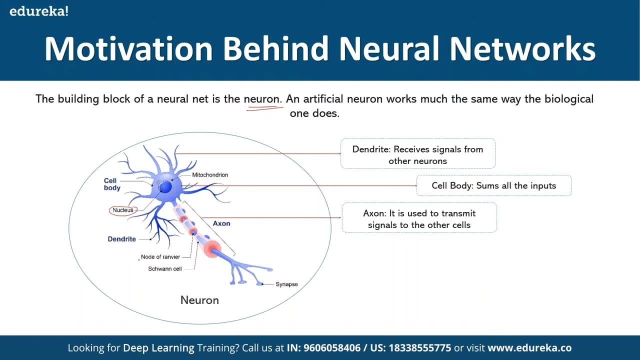 okay, and you know, it has something known as exon, okay, and these are known as dendrites, okay. so if you see a dendrite, what they do, they receive. so what happens in human brain? this is suppose this. this represents this image. this circle represents this image. just imagine, inside this we have this. 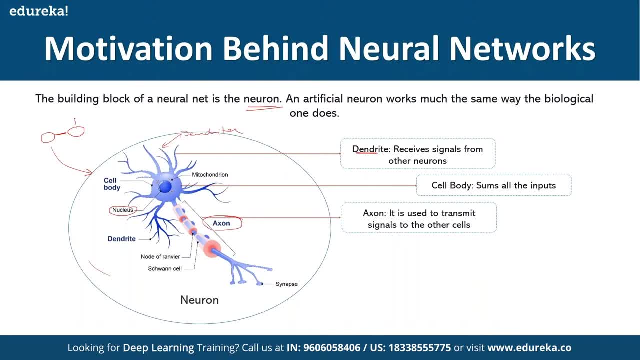 okay, not, this is connected to another. this, that is neurons. so there are neurons connected with other neurons, so there is a network of neurons. okay, these are connected with each other. how are they connected? they are connected using these dendrites. okay, now, once they receive an input, right once they receive. 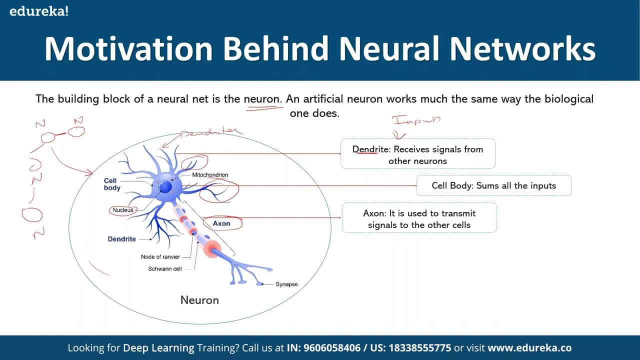 an input from these dendrites, they will process it in their nucleus or the cell body and they will give an output from them, and then they will give a〜 put using the axon. okay, so for example, suppose we listen to music. right, human, we listen to music. 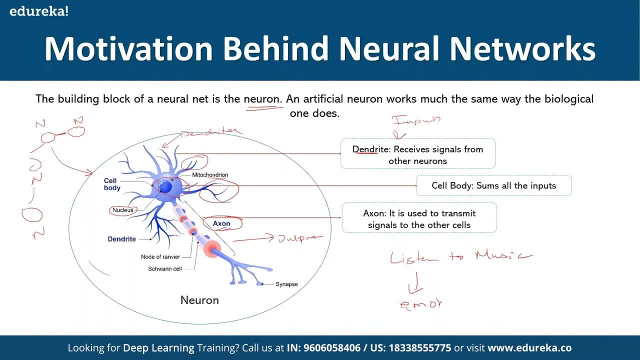 what happens. certain emotions are evoked, right, certain emotions are evoked. so the input to our brain is music right from our ears. so maybe yours are our sensors, from that we listen to music. the neurons, artificial neuro, sorry the neurons- they will process it and your mind will feel the 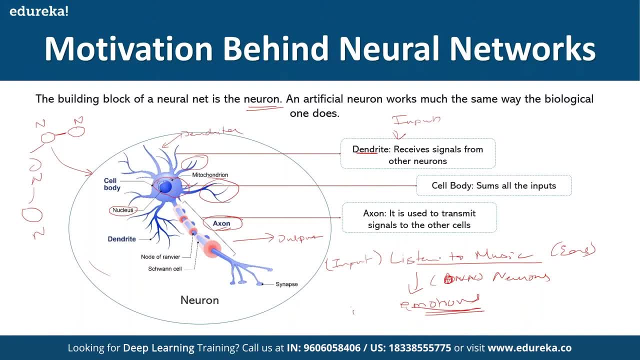 emotions. your body will feel the emotions right. but who is taking this input for you? the neurons are taking the input, and who? what is it giving you? it is giving you output. each neuron is connected to other neurons, and one and second is: each neuron receives the input and it gives the output. so what? 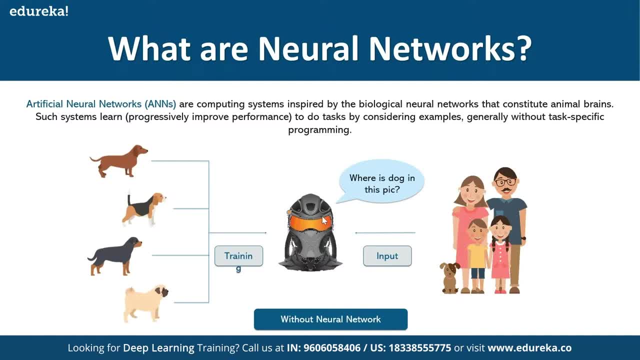 we need to learn about the body, how it is abuting theinary memories, right so how we learn about the neurons. and those neurons, as i said, summers, they have given birth answers, they have given us knowledge. next time, if there is an increase in the volume of our brain, inr 예�, just look for the active. 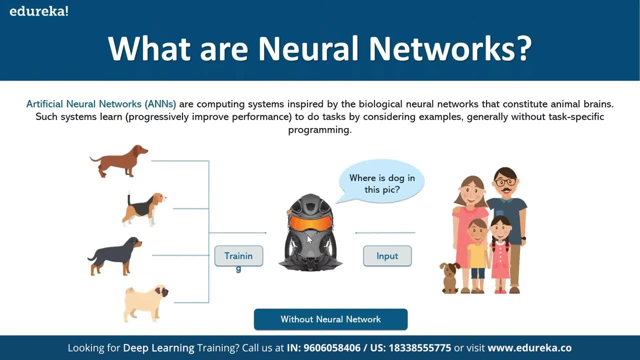 brain center and if your brain plays a plays a role, your brain will be active. you will get session from conversation and you will learn with that. the mind has to come up with ideas, like man has seen his friend telling him anything he wants. it is that mind. 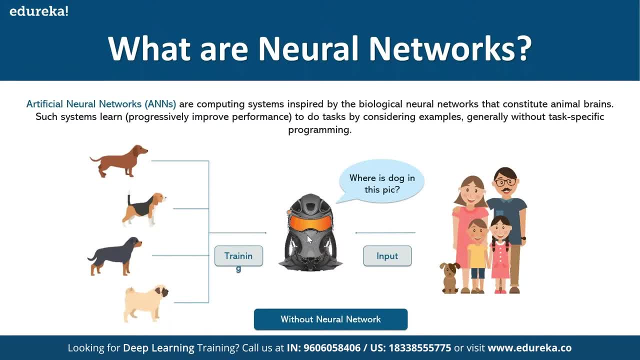 of man and head to pen også. yani here is another slide. mind has got trained that this person is my mother, this person is my father, right? So you have trained your mind to understand different relationships, different persons, different concepts, different voices. even smell can make you identify. Similarly here what we. 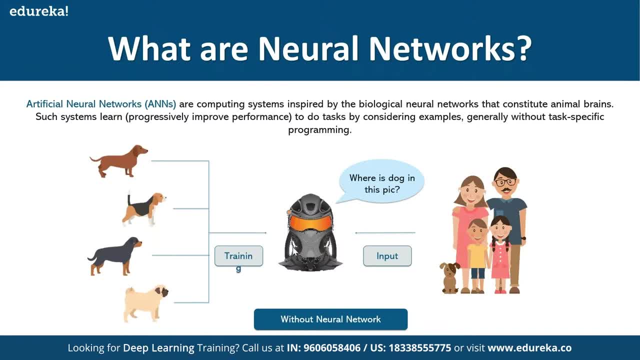 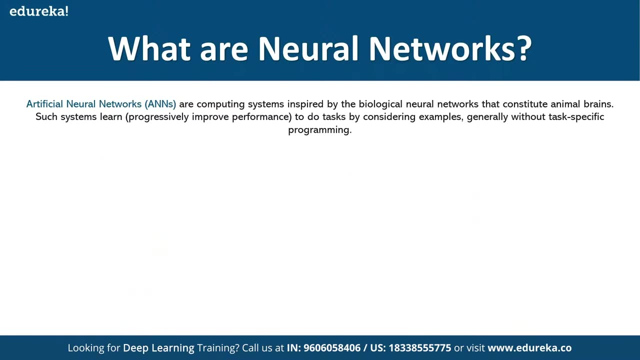 are trying to show you here is if your mind doesn't have neurons and suppose you see some human beings, right, But you're only seeing the dogs. you're not seeing the other parts. why? Because your mind has not been trained right. So, if you see, if I ask the robot, 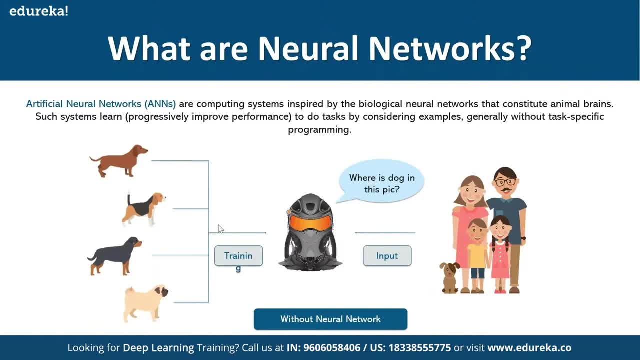 where is the dog in this pic? Where is the dog in this pic? So suppose you see a mobile right In your mobile, your mobile can see where your faces are right. You know autofocus things are there. Similarly here, suppose you want to understand with your camera where the dog is, please. 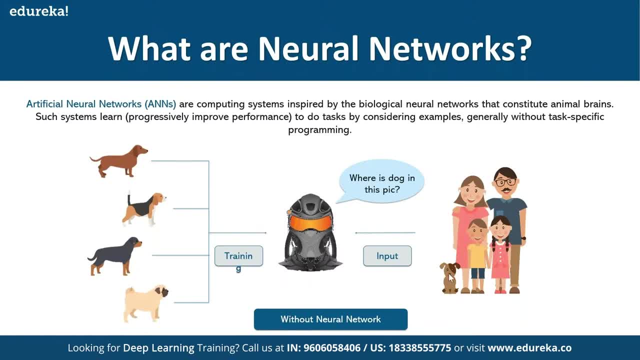 locate the dog. If it is not trained for that it will not be able to locate. But if we train this neural network with different dog images, then after training it will be able to say: okay, there is one dog in this pic. It will identify: okay, there is one dog in this pic. 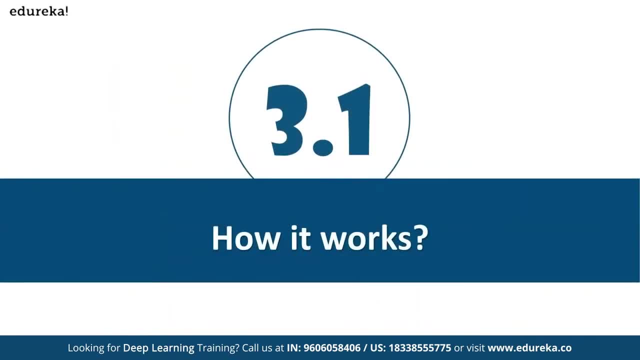 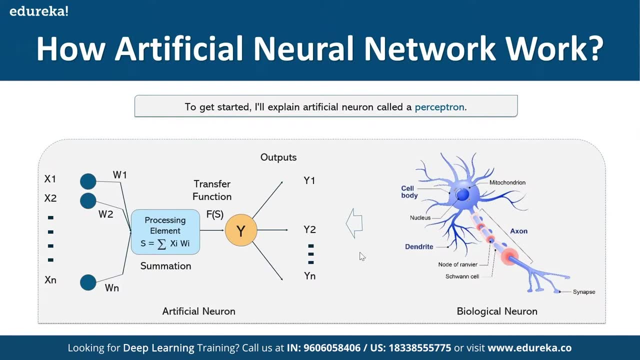 Okay, So let us try. So let us try to now understand how it works. So similar to this biological neuron, we have created now this artificial neuron. Okay, What does it consist of? It consists of three important things. One is input, which is represented. 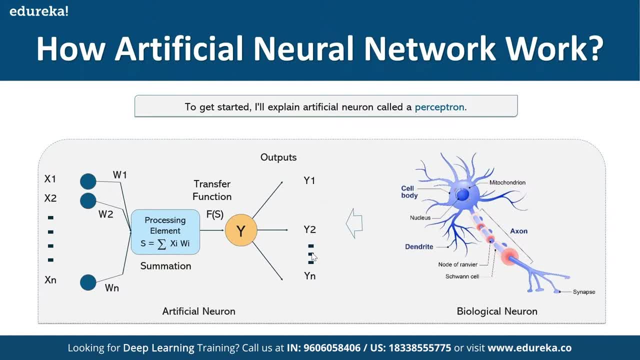 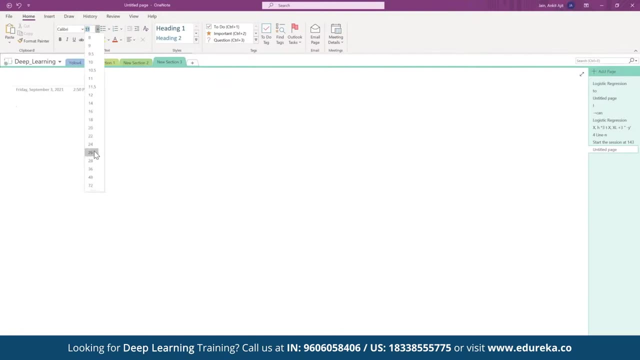 by X, One is output, which is represented by Y And there is a transfer function in between. transfer function in between. Okay, So if I have to list what are the important things you need to understand, The important things you need to understand here are input, output, weights and a transfer function. 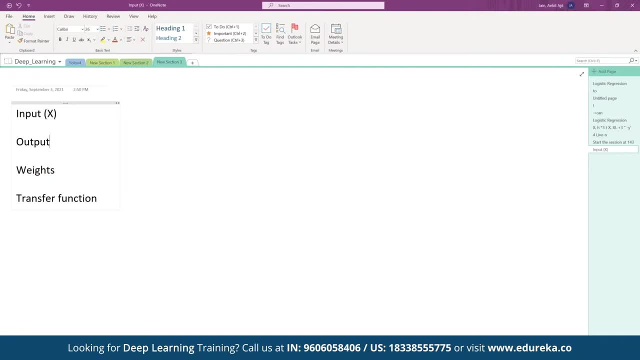 So input is represented by X, Output is represented by small y, Weights are represented by small w or capital W, And transfer function is a. transfer function is a equation which I will explain to you, Okay. So again, what happens is: let me give you a practical understanding. 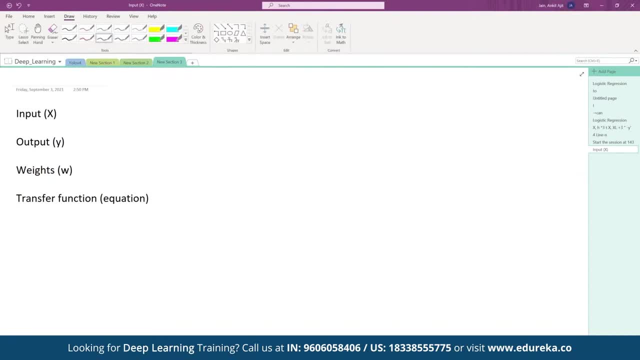 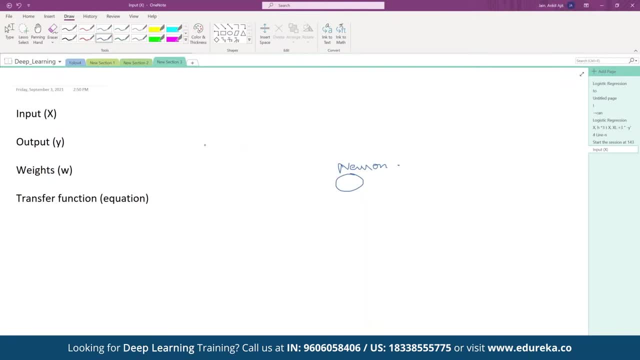 Okay, Okay, Okay. This is your neuron. Okay, And now I am giving an input to your brain. Welcome to Edureka. Okay, Now three words will go into your neuron, right From your ear. it will go to your neuron. 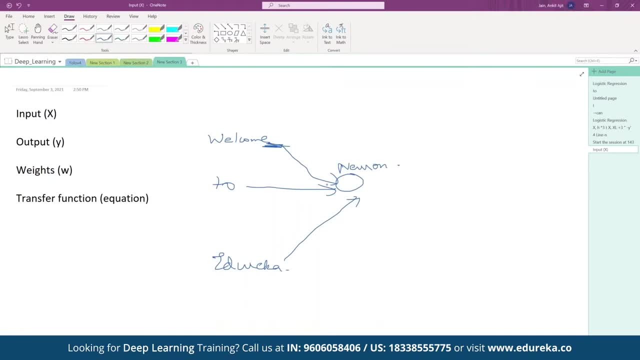 So what are these? Welcome to Edureka. These are your input. X To the face. X raise your hand. that x Welcome to Edureka. X, imagine this data. it is an input to your brain. Okay, Now, in this, suppose I say which: 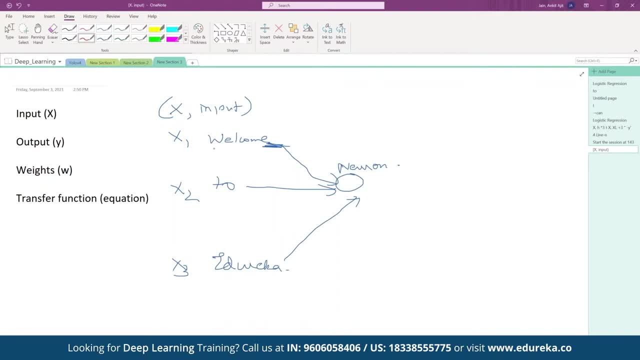 are the important word here, which is the most important word. are all the words more important here? No, the most important word is welcome. Okay, Correct. So what will be output from this? your output will be what your output will be you. you will also say thank you. 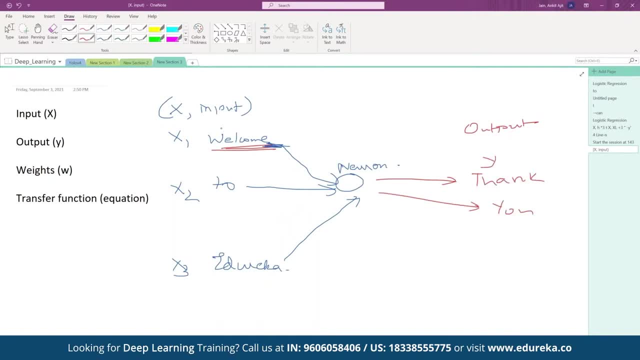 correct. now. when will you say thank you? when you will listen to the word welcome, right, so most important word is welcome and the second important word is edureka. the third least important word is two. right, so all the words are not equally important. here there are some weights associated. 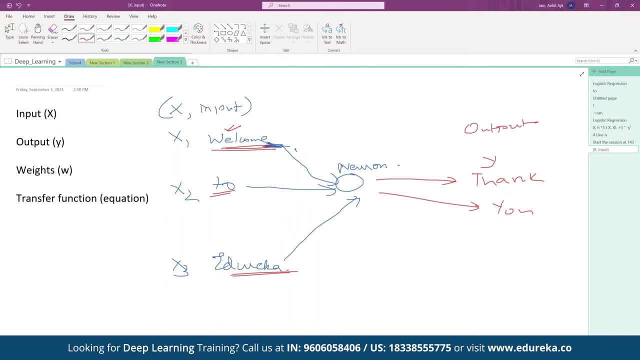 with it. so the neurons will receive this input with some weights. okay, so suppose i say this is w1, this is w2, this is w3. input is given, some weights are associated with it, right? so total, total information which goes to a neuron are what it is. total information which goes to a neuron is: 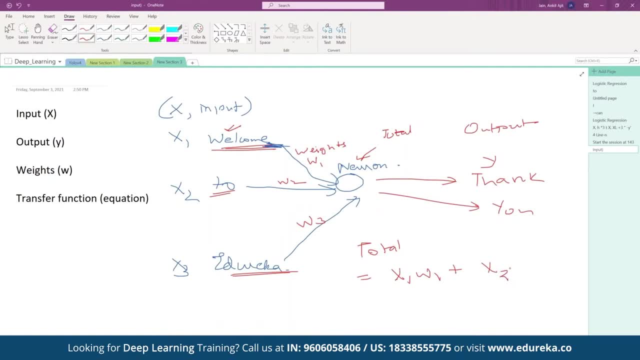 x1, w1 plus x2, w2 plus x3, w3. okay, so these are the three inputs, three weights. total information is the product of them plus addition of them. so this is what goes to a neuron. now, what does this neuron do? it will process this information, this total information. what it will do? it will process it. 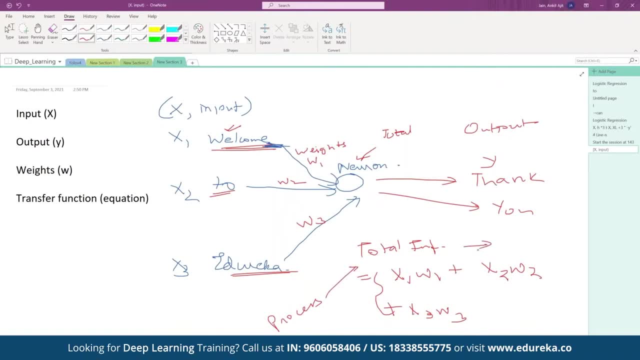 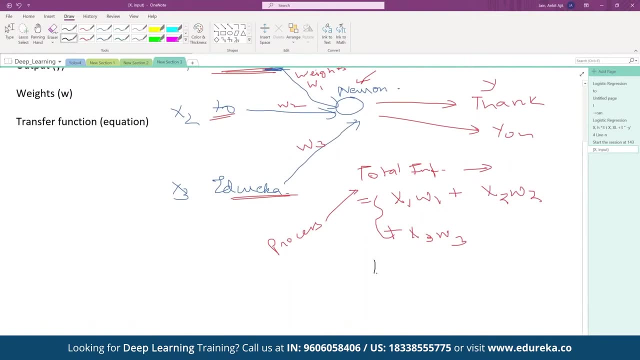 it will process the total information. okay, how will it do that? we run this, the every output will be: change the value to a with a small one. so what do we do here? we apply the total information. it will process by applying a transfer function. so, just as our brain does some calculation, we will apply some. 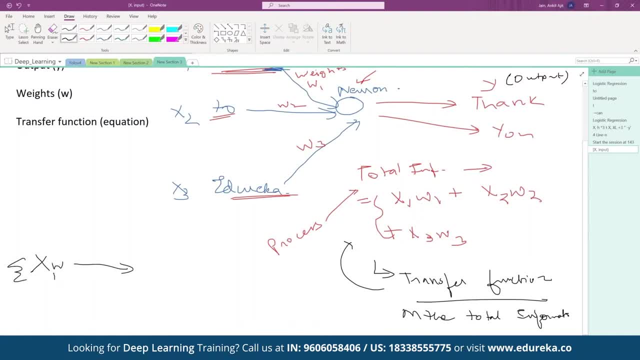 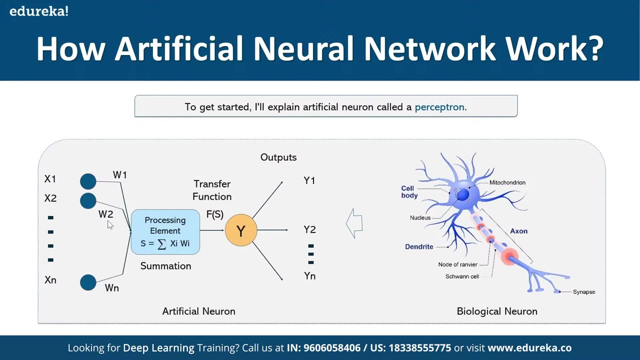 transfer function on the total information: Sigma X, I, W, I we apply a transfer function to it and it will give you out: okay, so this exactly is given here. we have an input, we apply W weights, we we do the summation of the total information, we apply a transfer function. 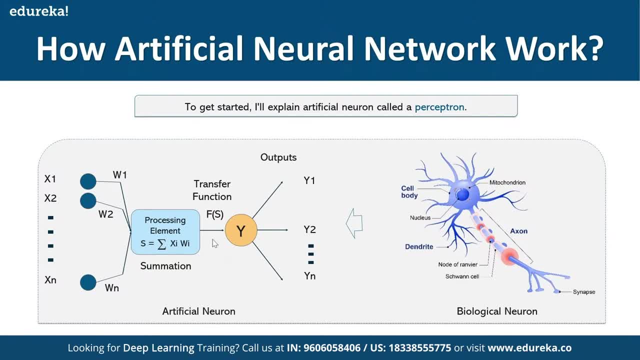 FS and we get the output Y. now what is this transfer function? we will understand that. for now, just up, just understand that there is a transfer function applied. okay, so this is why it is called artificial neural network or artificial neuron. the reason is it mimics the biological neuron. it mimics 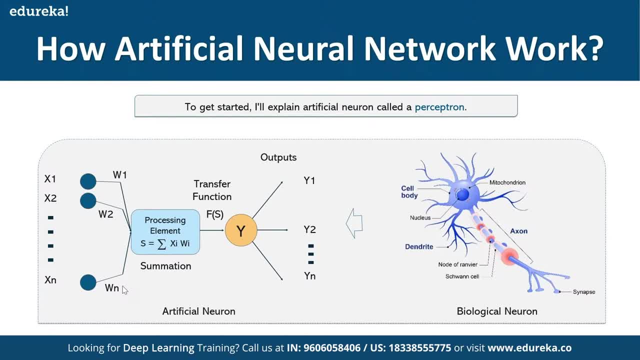 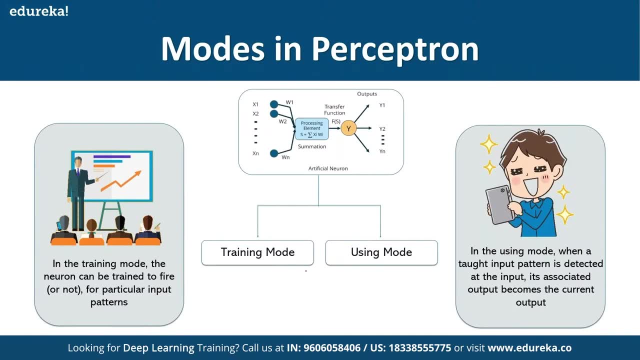 the biological neuron. therefore it is known as artificial neuron. now how can you use this neuron? right, so that neuron works in two modes: training mode and using the neural network. so this is why it is called artificial neural network mode. in the training mode, what happens is the weights are locked. we will lock. 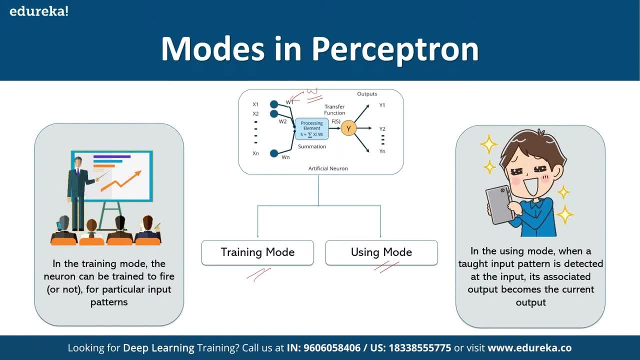 the weights and in the using mode. we will not change the weight. we will use the neuron as it is to make it more interactive for you. to make it more interactive for you, it is something like this: once you recognize that, suppose my, my name is Ankit, right? suppose you recognize that. 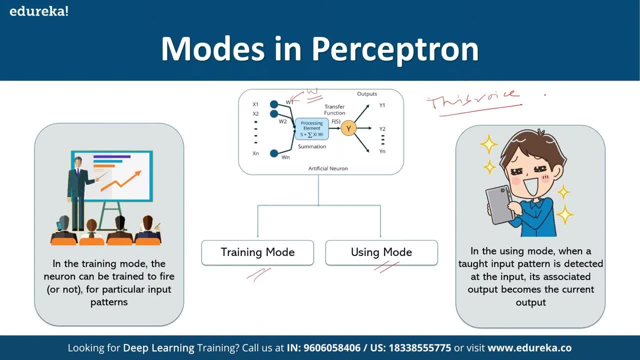 this voice today you heard it for the first time. right, it represents Ankit. now your mind knows that. okay, the voice I am listening to his own kid. now that is your training mode. you are being trained, right, so one hour you will listen to me, you're. 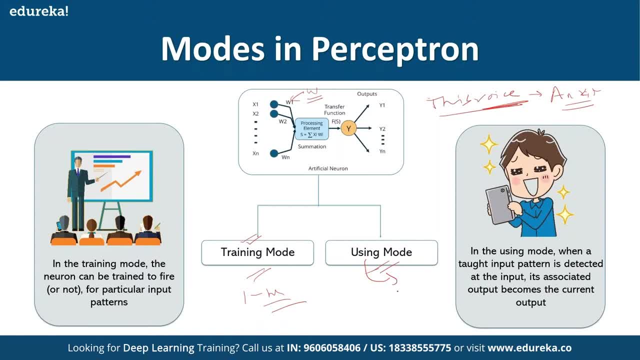 getting trained. today, the next time I, if I come and speak to you right, you will not be required to trade. your weights will be locked right because you have already been trained with my voice. now, next time when I come here, you're already, I don't need to introduce myself. 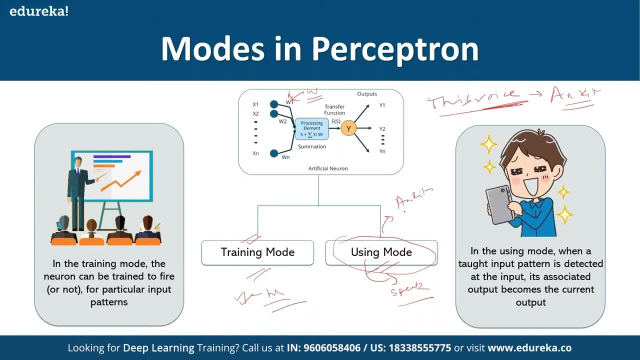 As soon as you listen to my voice, you will say it is Ankit speaking. right? This is how we identify most of the actors, right? We understand who it is by their voice, also because we have been trained to listen to them, right? 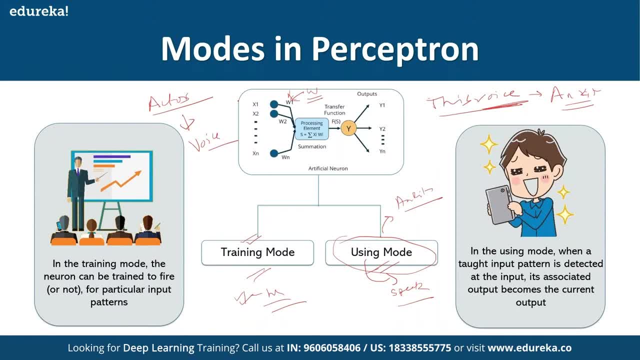 Similarly, our parents are all known. right, They are trained. So when we see modulation in our voices- right, They understand what emotions you are going through. right, Are you tensed, Are you feeling worried, Are you happy? right. 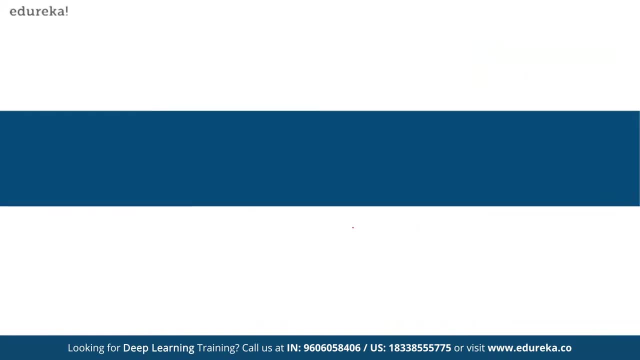 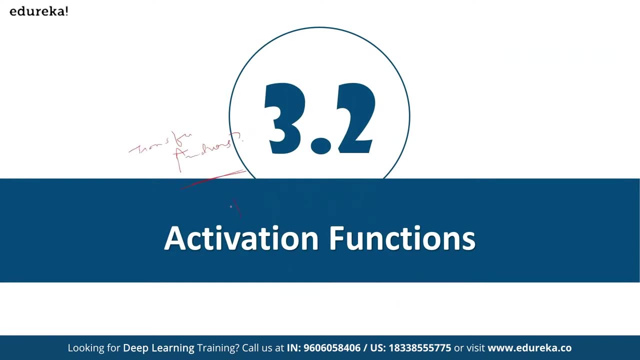 So that is the training mode and the other is using mode. okay, Now what are transfer functions? We'll come to that. okay, So transfer functions are also known as activation functions. Is it clear? Transfer functions are also known as activation functions. 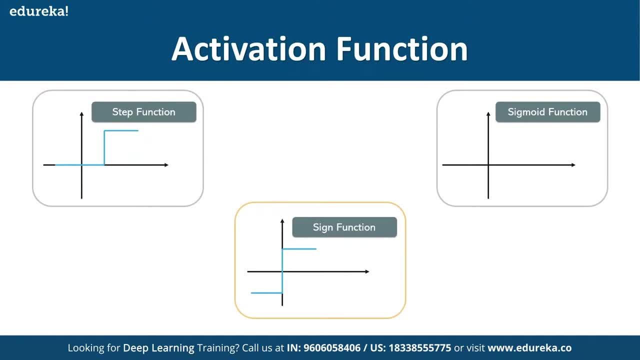 Now what kind of transfer function we apply. We basically apply a math part to it. We may apply a step. So whatever information you are getting, always remember we apply activation function on the total information. So whatever information you are receiving, you will apply either a step function, a sigmoid function or a sine function or some other functions. 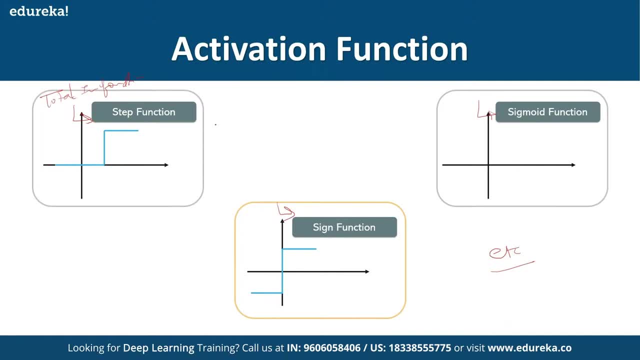 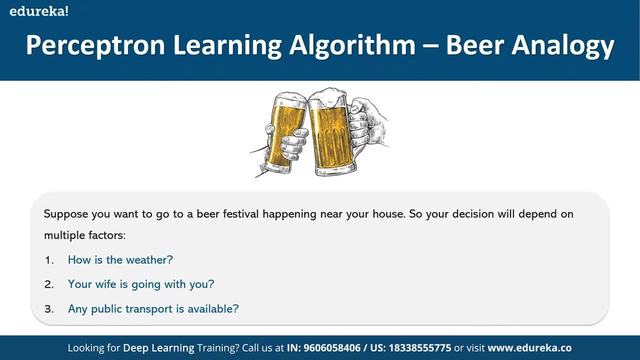 So, basically, your information comes and you have a function applied to it. I'll give you some practical understanding. So let's first try to understand this. Suppose you want to go to a beer festival happening near your home. What will be your decision, depending on whether you will go there or not? 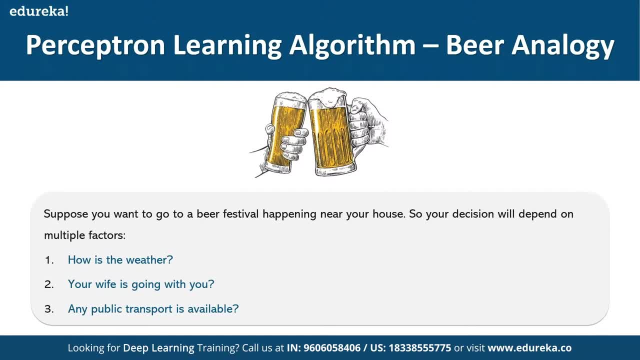 It depends on how the weather is right. If you are going to a beer festival, you may want the weather to be conducive so that you can consume your beer. You can enjoy the beer right, But if the weathers are not conducive you will not go. 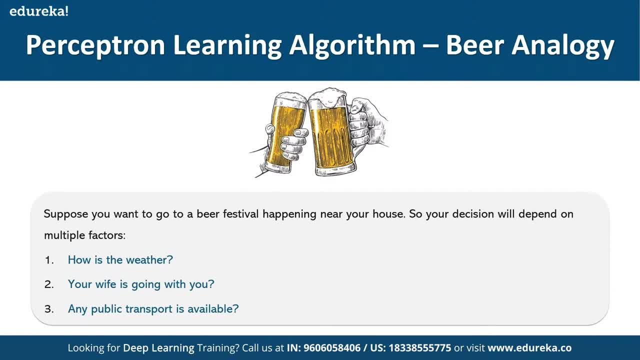 So first is weather, Second is who is accompanying you. Is your wife going with you? Are your friends going with you? So that is another important factor. And third is what the weather offers. transport you can use to go to the beer, function right. So can you go by a car or you will take a. 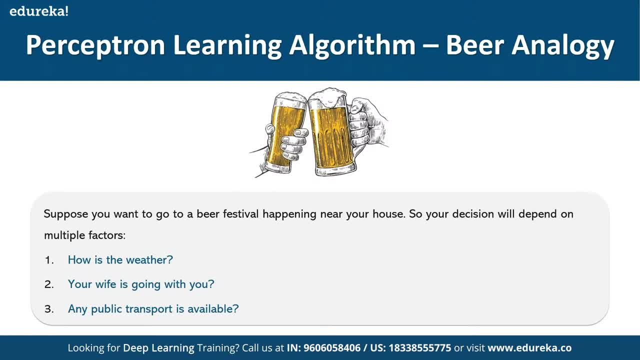 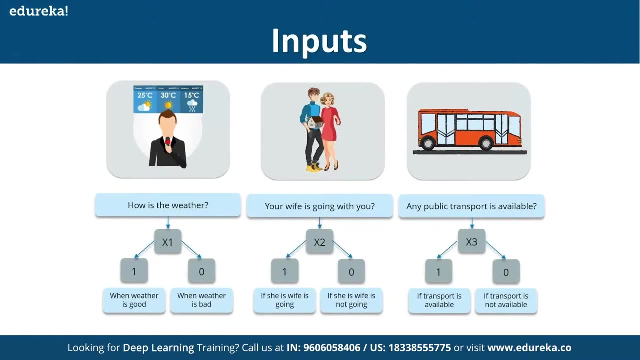 public transport: right. So, based on multiple factors, you will take a decision whether you should go to the beer festival or not, right? So let us first try to understand each of the parameters So your mind will understand. how is the weather? x1.. So the first input is x1.. 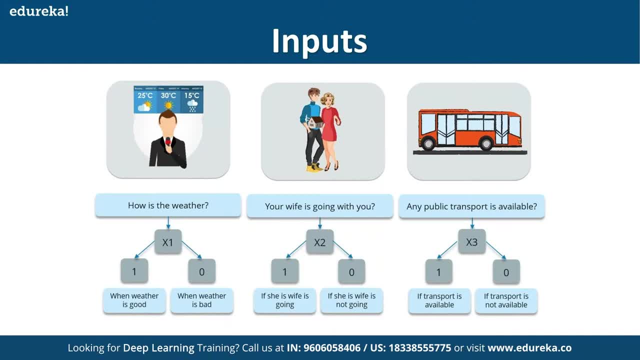 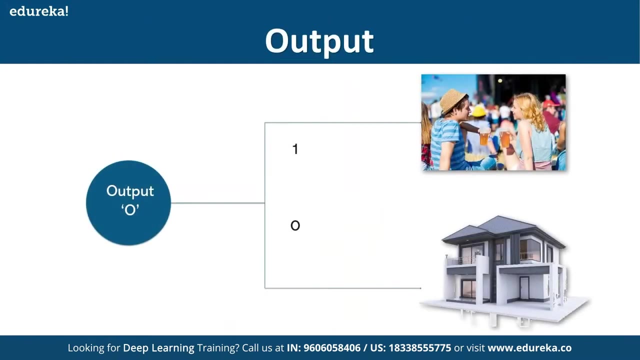 If it is 1,, it indicates whether it is good. If it is 0,, it indicates whether it is bad. Your wife is going with you. x2 is your second input. Is it yes or no? Public transport is available? yes or no? That is your third input, And what is your output? Yes, you may go to the 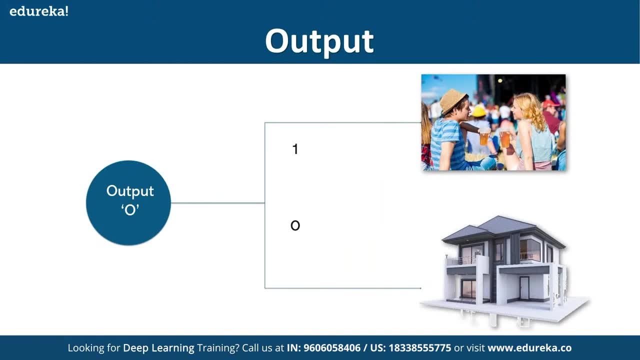 beer festival or 0,. you may not go to the beer festival. you may remain at your home right. So the possibilities are clear for everyone. Input are x1, x2, x3.. Three inputs are possible: x1,, x2, x3.. Three inputs are possible And in every input you have either 0 or 1, right. 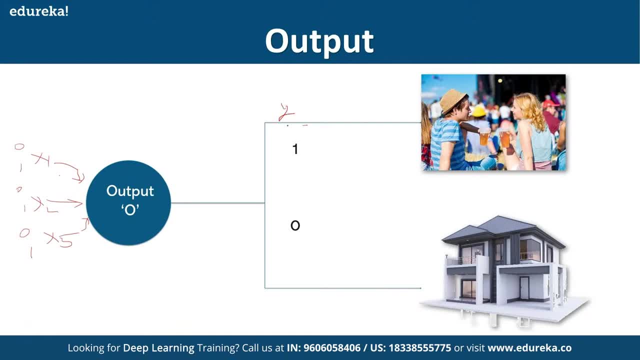 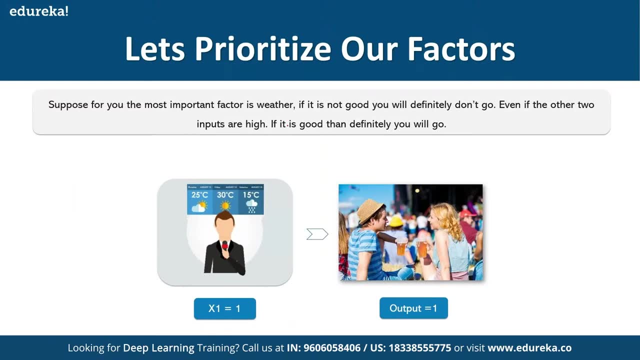 And output is also 0 or 1, that is represented by y. Now let us prioritize our factors. So the first factor is: the weather should be good. x1 is equal to, then for sure your output is 1, right, If weather is not good, obviously you will never go. 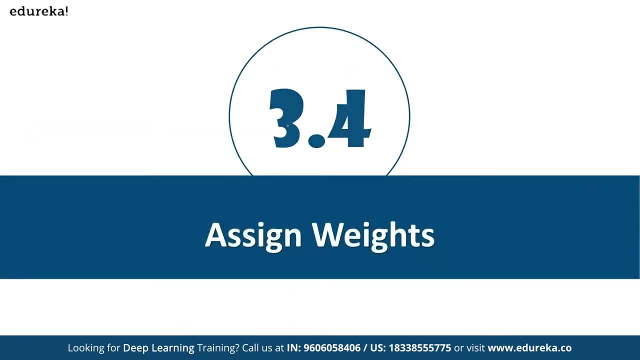 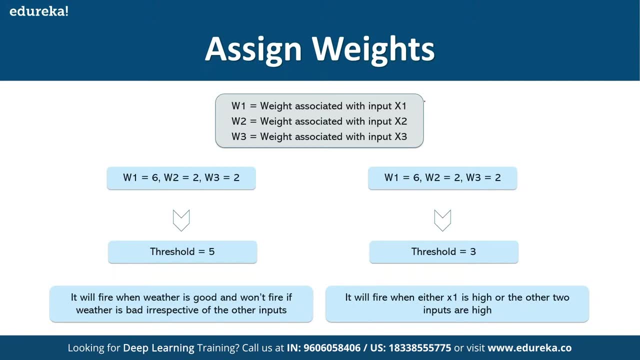 But if the weather is good you will go. Then we will assign the weights. So, according to each factor, we will assign the weights, For example, weight associated with x1, weight associated with x2, weights associated with x3. So these three weights- say example 623 or 622, it will give you. 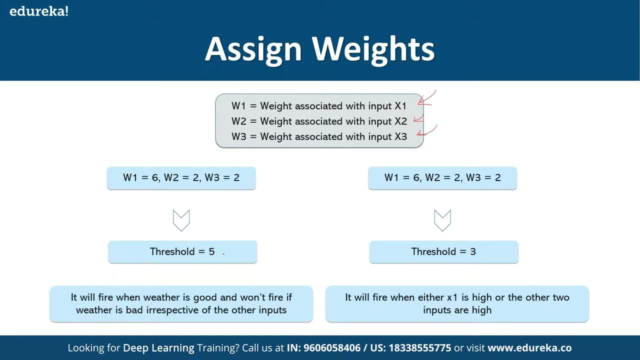 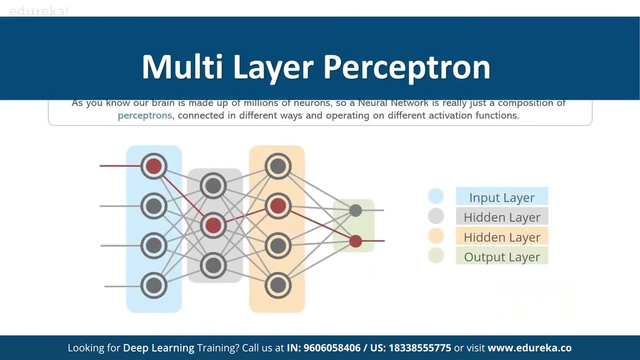 total information And, depending on total information, if it is greater than 5, then you will go. If it is less than 5, you will not go. So there is a threshold there. that how much is the threshold reached when you apply weight to your information? Now, as I said, one neuron will consist of: 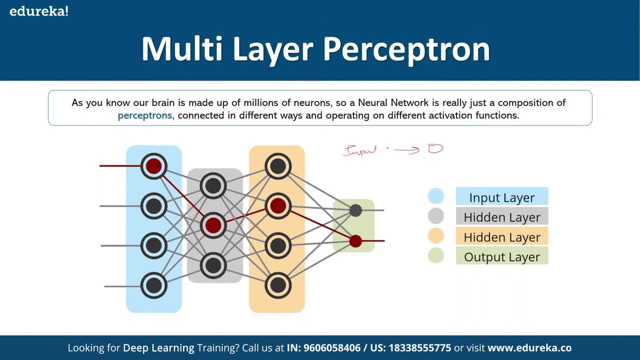 these things? What Input, right? You have transfer function or activation function applied to it And then you get an output. What Right? So this is what happens in a single neuron. Now, each neuron is connected to each other. So if you see a human brain, right, You can see four neurons are connected. 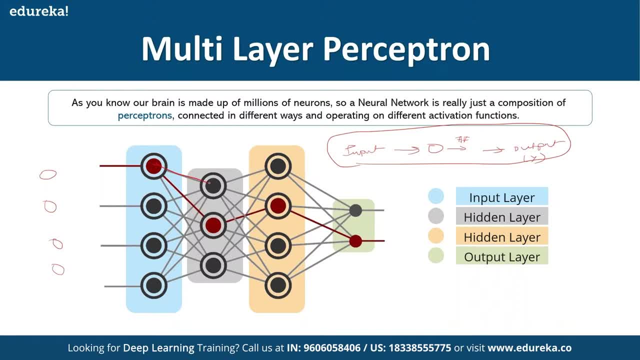 to three neurons. Now it is not like this neuron will only be connected with this neuron. No, it will be connected with other neurons also. So can you all imagine now the complexity of your brain. Every neuron has weights. So if you see here 1w1, w2, w3, w4, input weights Similarly in your mid-layer. 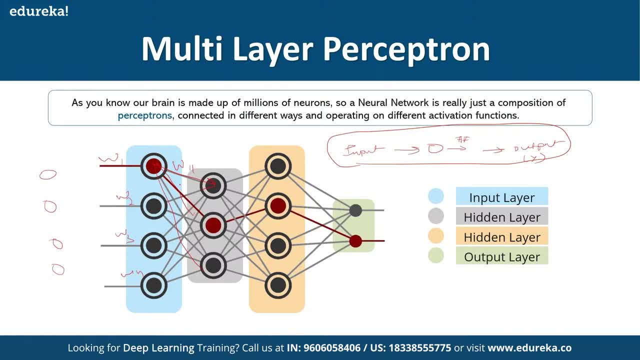 you will have weights associated with each neuron: w11,, w12, right, It is also going to w13.. So total nine connections will be here, right, And then each three is connected to four other neurons. So these neurons in between, 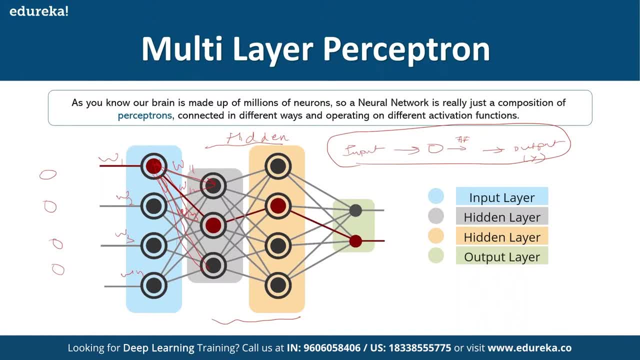 are known as hidden layers. This neuron is known as input layer And this is known as output layer. Can you all imagine now, it is your human brain, where each neuron, every neuron, is connected to each other? Okay, so, which is the hidden? which is the input layer? the blue one you can see here. These are: 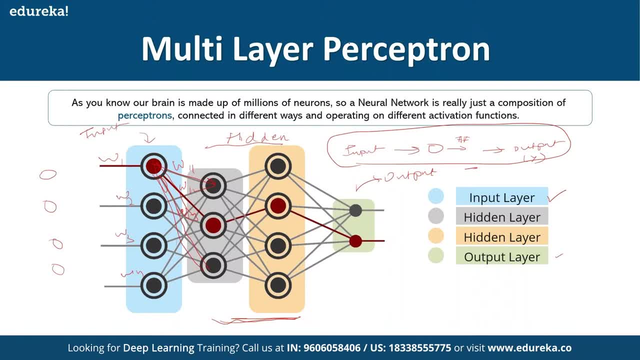 your hidden layers and this is your output layer. now i can explain you the term deep learning. you may have heard about it, right, deep learning. so deep learning is nothing but a neural network in which your hidden layers. a deep learning is nothing but your neural network is greater than one. so if your neural 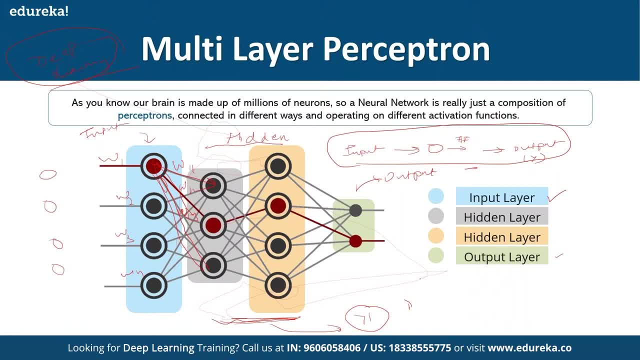 if your hidden layers are greater than one. we call it deep learning. i hope you are able to associate yourself. not the deep part is because you are learning, trying to learn deeper. you are having more layers between input and output. you are giving more thought to your process. 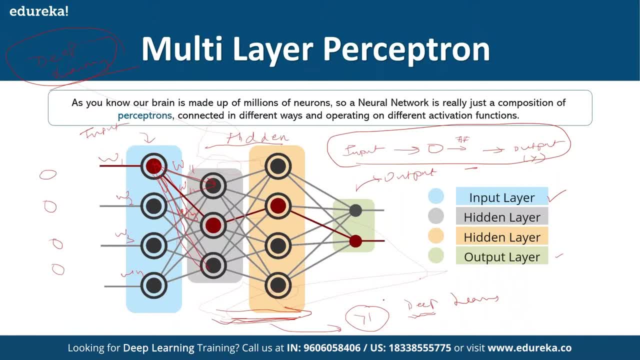 more process to your thought. and second is you are learning through this artificial neural network. that's why it is known as deep learning. okay, the hidden layers, where we apply the function and the number of neurons. yes, in the hidden layers also we apply transfer functions. so every neuron, you will see, there is a transfer function after it. 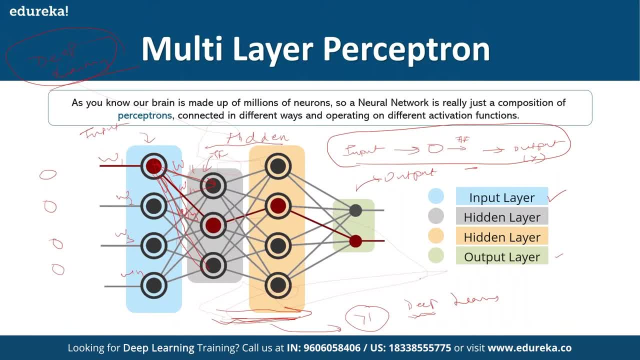 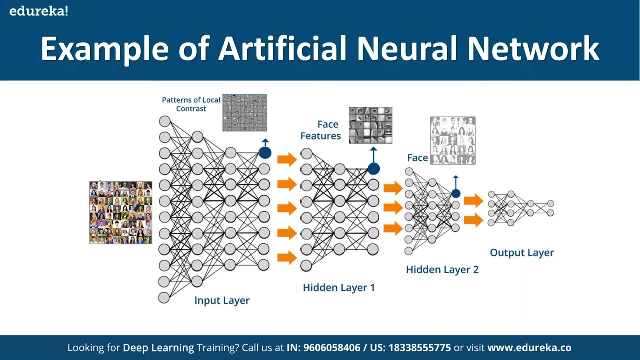 and there can be more neurons. you can have hundreds of neurons in a single layer and there can be multiple hidden layers. you can have two, three, five, ten, whatever you want. so this you will see examples. suppose you want to process each of the faces on this image. 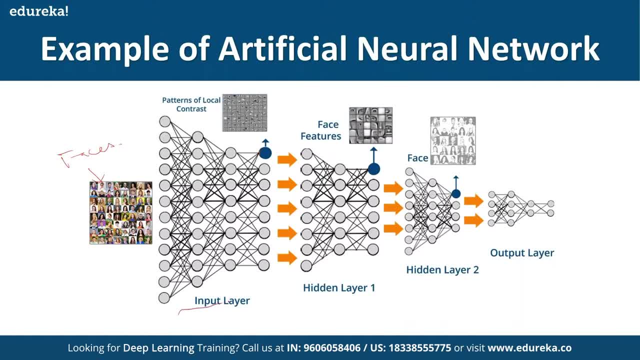 okay, what you will do: you will pass it through various input layers, you will pass it through hidden layers and then you will get a output layer. so here it is, showing that, after, after doing some, you know- manipulation over this data. this is how this image will look. this is how it will look. 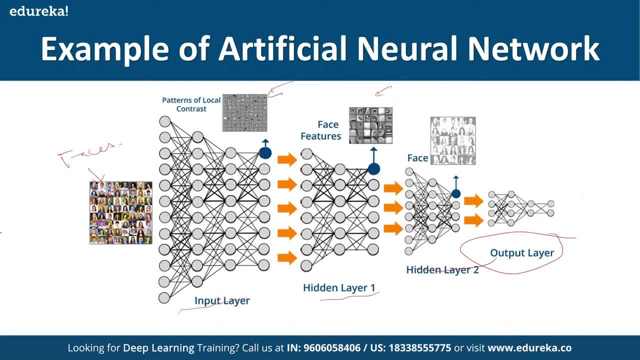 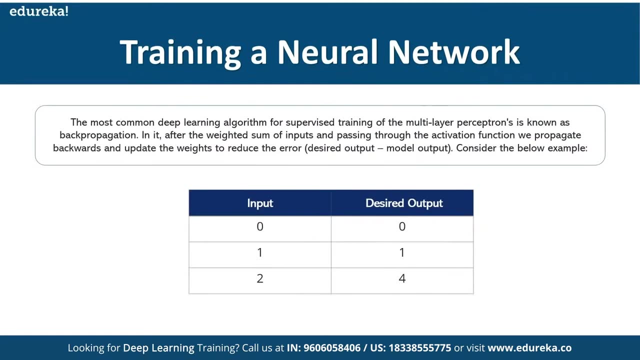 at the end, after the output, you will be able to see, okay, each image. you will be able to identify who is there in that image, okay, so such kind of complex neural networks we have to develop. now, how do we train a neural network? so we train the neural network? for this, there is a concept known as supervised learning. what is it? 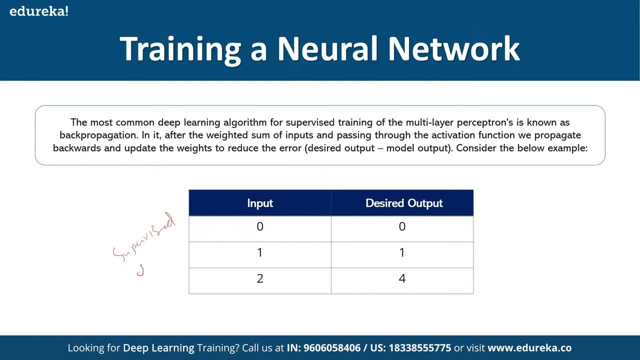 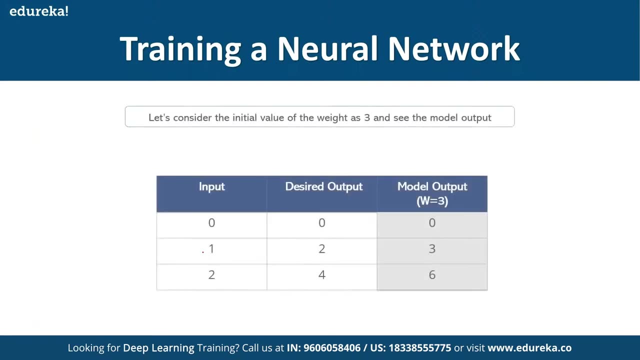 known as supervised learning. now, in supervised learning, what happens? you have an input and you have an output. so there is an input layer and there is an output layer. and what will your model do? your model will assign the weights to it, so this happens. this is your. 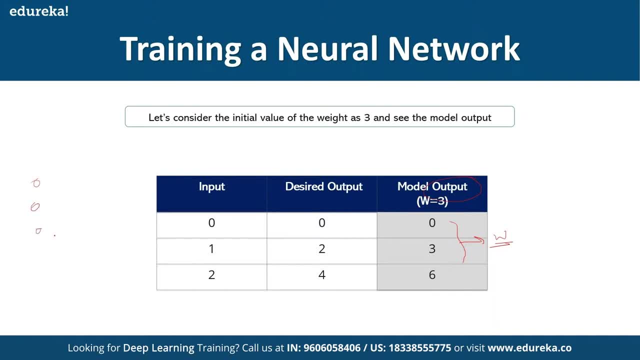 model output. so you have your input and you have your output. in between, say, you have one hidden layer. now every neuron is connected to other neuron and there is a weight associated with it. who will assign this weight? this weights will be assigned after you do training of this, after your. 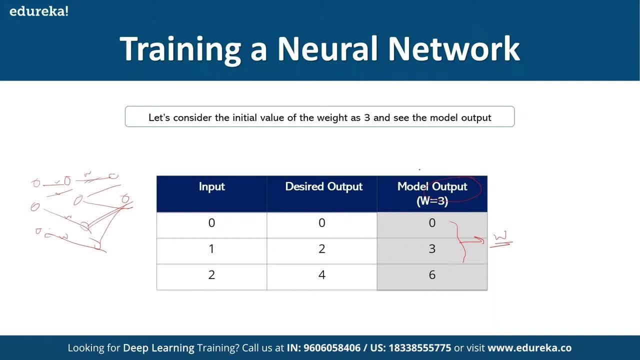 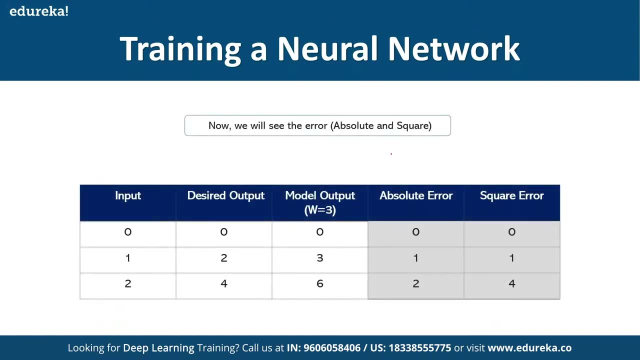 training has been done, these weights will be associated, identified by a model. that will be your model output. okay, so what happens? initially, you have a input, you want output of zero and you have a model output of zero. here, your input was one, desired output is two. but what did your model? 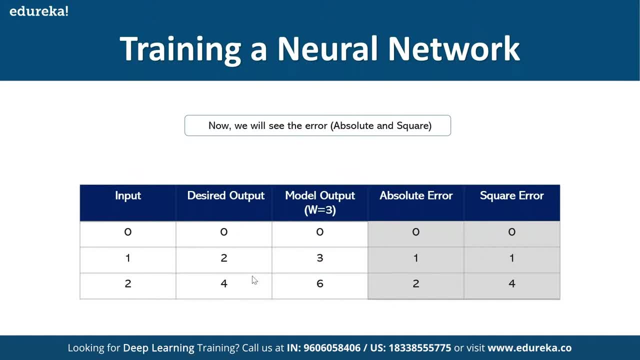 give. your model gave three. here it was two. your model output is four. So if you see, your input and output are double of each other. but here, what your, what your model or neural network is giving you are giving an input, it is returning value of three. So there, 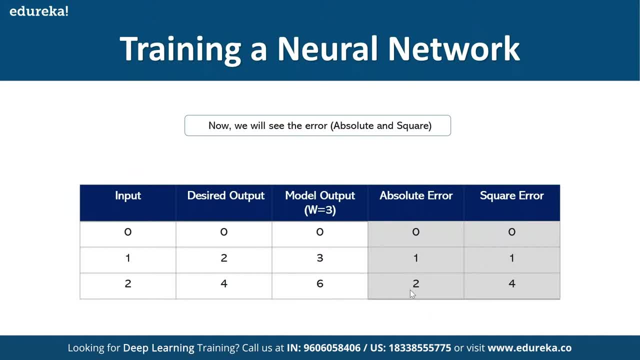 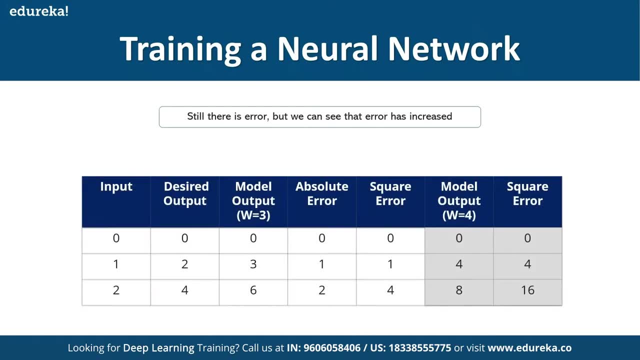 is a difference of one right error, of one error of two. So what it will try to do is, basically, it will try to minimize this error. okay, it will try to minimize this error by adjusting the weights. So if you see, as in, when it adjusts the weights you start, so suppose you now keep a weight of. 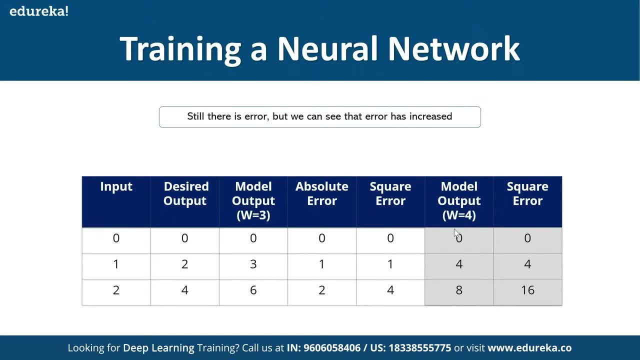 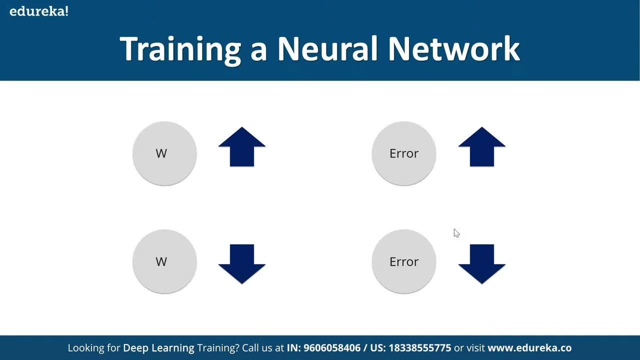 four instead of three. this is the values you are getting right. So this way it will do changes in the weights of your neural network so that your error can reduce. So if you see at one point of time the weights right, at one point of time the weight at particular. 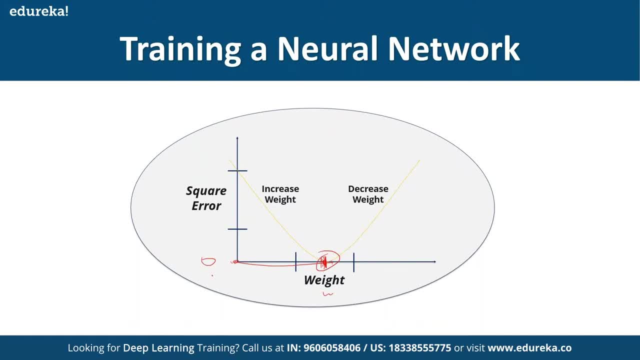 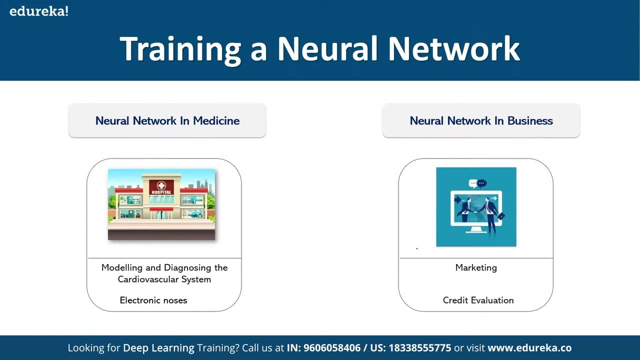 range. So this is the weight value. your errors are zero. your errors are zero. this is the weight of your neurons which will be locked. So where are the neurons used? neural network use. the neural networks are used in medicine, in business. it is used everywhere. okay, So your Alexa. 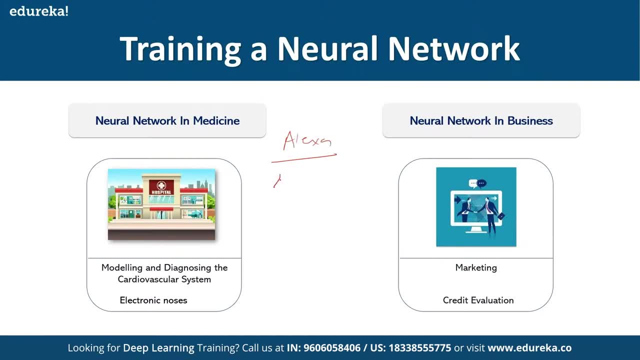 okay, all your you know face recognition technologies. okay, all your you know face recognition technologies. all of them are using neural network based models. okay, So suppose you give a x-ray? okay, suppose you give a CT scan and your model will detect whether it is a COVID or not. okay, So this model usually 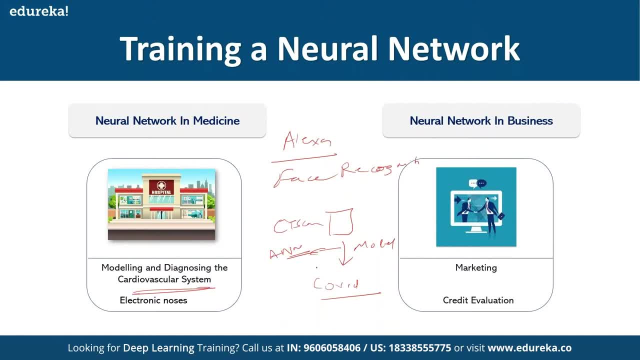 are artificial neural networks. so it is used in a lot that electronic noses. now you have, you know, sensors which can sense the smell, Which can sense the smell for use it, a good smell, bad smell, in hospitals and all. so those sensors, artificial sensor, are also using artificial neural networks. Similarly in business, for marketing, for. 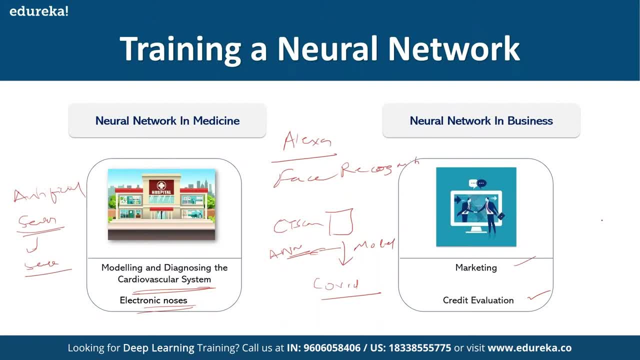 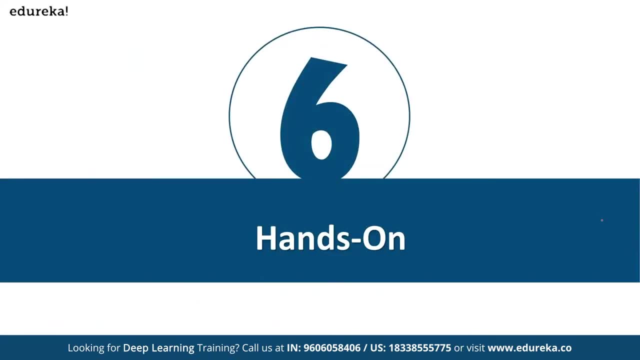 credit evaluation, whether you should give that person the load or not. all these things you will get using neural networks. So let us do a hands-on session now. let us try to create a neural network. So what we will do for that, for hands-on session. let us try to create a neural network. so what we 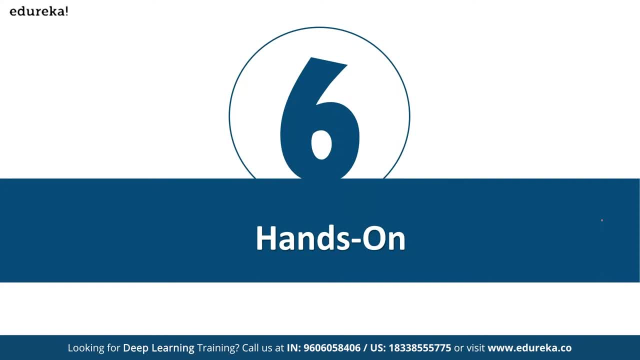 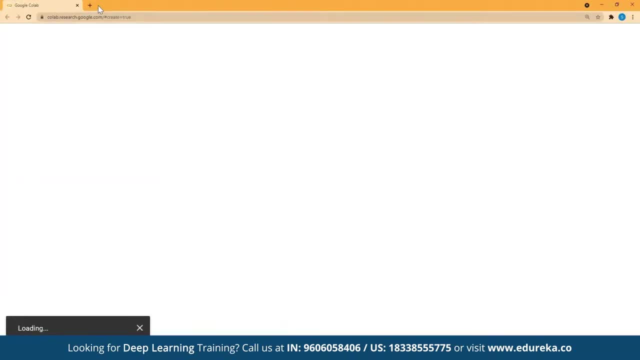 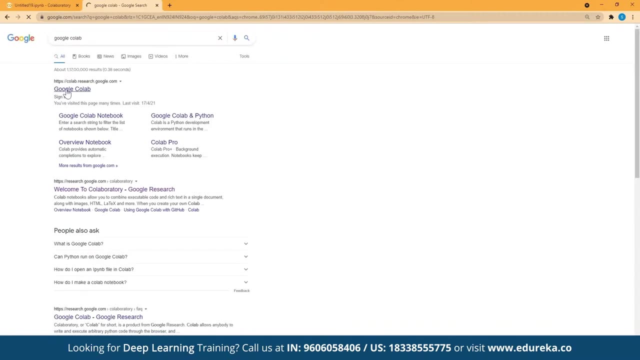 on session. we will use a platform. okay, we will use a platform known as colab. all of you, you can open google colab. so if you search online google colab, if you have a gmail id, okay, you can open this google colab. okay, now in this colab, what happens is you can create: 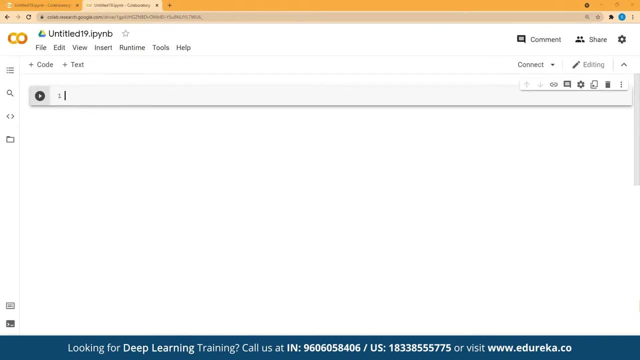 a notebook. okay, you can create a notebook and in this notebook it is like a laptop itself. okay, so online on cloud. uh, google has provided you a laptop, a virtual laptop, which you can use for coding, so it has installed python for you, it has installed all the requirements for you know doing. 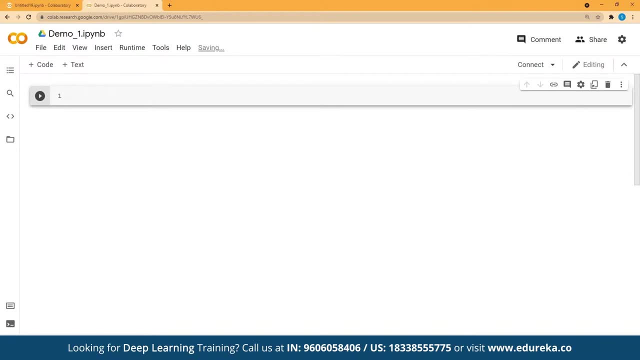 python, coding, etc. everything has been provided to you here, okay, so here, what we are going to do now is we are going to create an artificial neural network. okay, we are going to create an artificial neural network which will detect whether in the image, what number is there? okay, for example, i want: 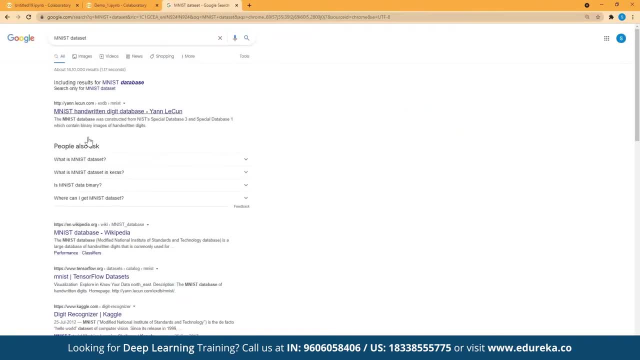 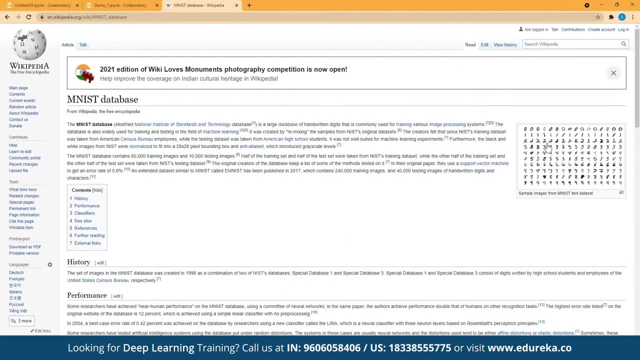 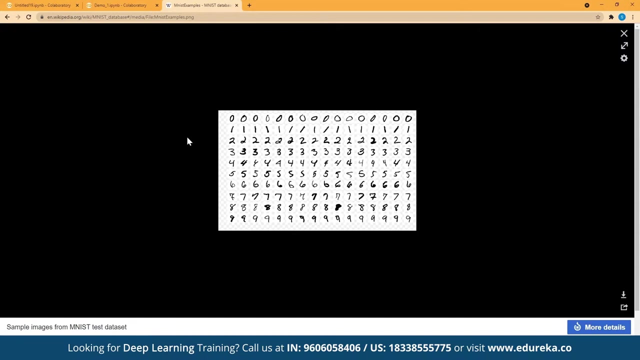 to create a neural network. what it will do is you will train the neural network with images. so, for example, these are the images, okay, and i will train a neural network which which will read these images and it will show you that on a particular image, it is 0, 1, 2, 3, 4, so it is handwritten. 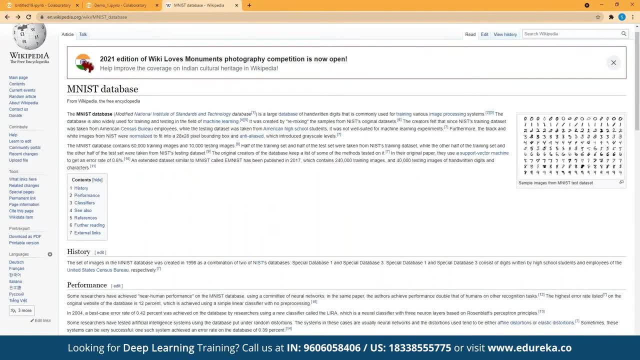 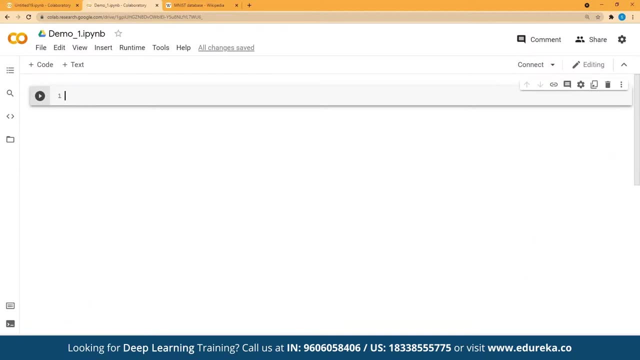 but it will also understand that what number is written on the image. okay, so for, in order to train that model, we already have a mnist data set which we will be using here. okay, we will be using the mnist data set. okay, so first, what we need to do. we need to import quite a bit of models in quite a bit of packages. 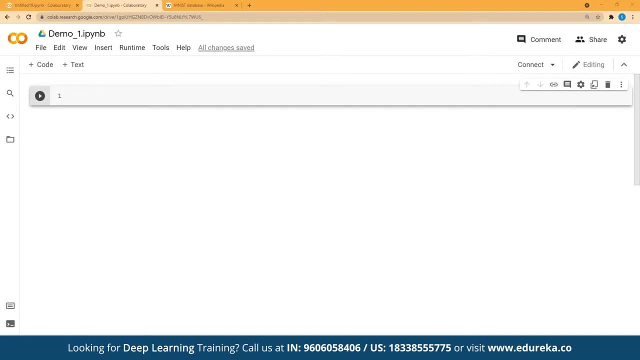 okay, so i am just going to give you what packages we are going to use here. so we are going to use for coding, which you will learn in detail if you go for the course or you do some structured calls. you will learn a package known as keras. what keras does is it uses. 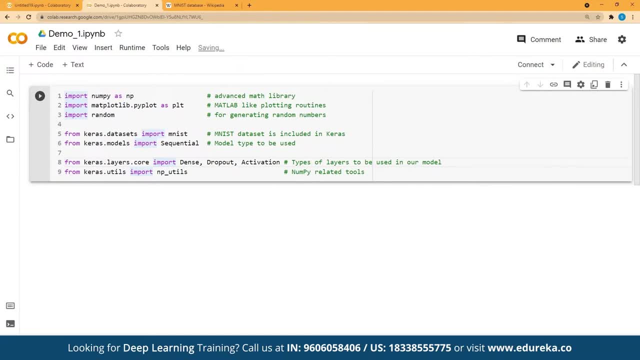 something known as tensorflow, in order to create your neural network. i will explain you with the demo. it may get somewhat clearer to you. so we are going to import all these packages. so these packages have pre-built in. uh, you know, we can create neural networks using these packages. 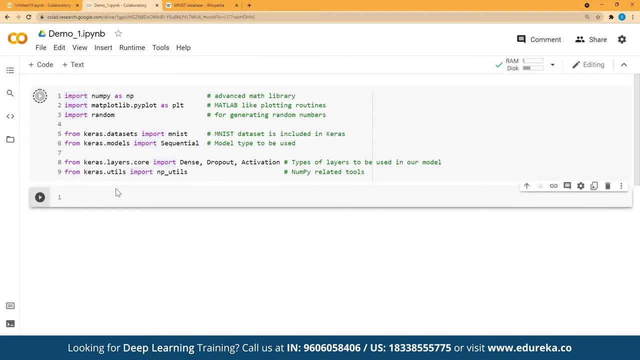 so we don't need to. you know, do, uh, write all the algorithms. it is pre-built. and what is the advantage of using collab here? all these in have been installed inside collab, so we are going to use a package known as keras in order to create a deep learning model. okay, so first, what i will do. 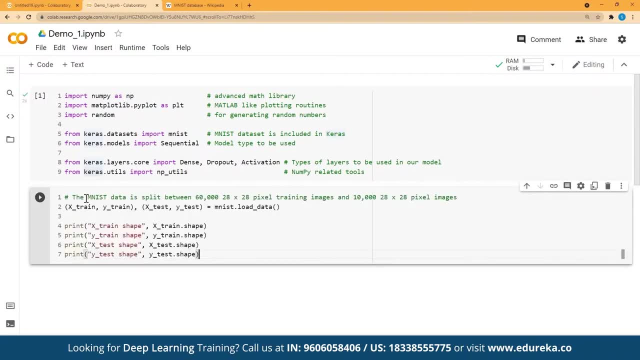 i will load the data set. the data set i'm going to load is the mnist data set, as i explained, mnist, what it contains. it contains 60 000 images, okay, whose size is 28, cross 28. these images, we are going to train on an artificial neural network and it will predict what is the number. 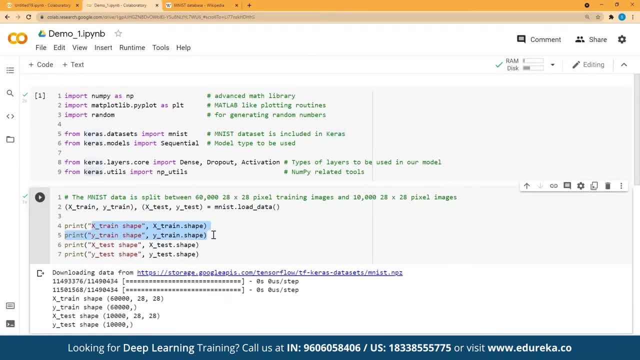 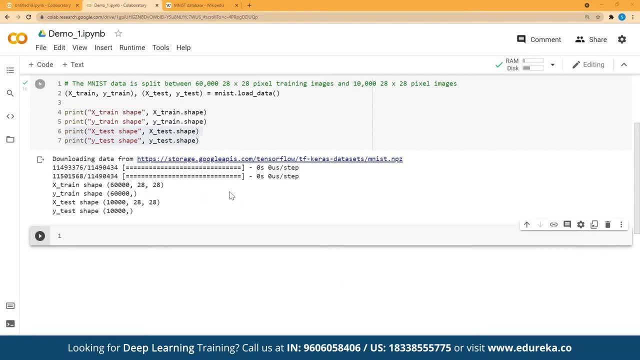 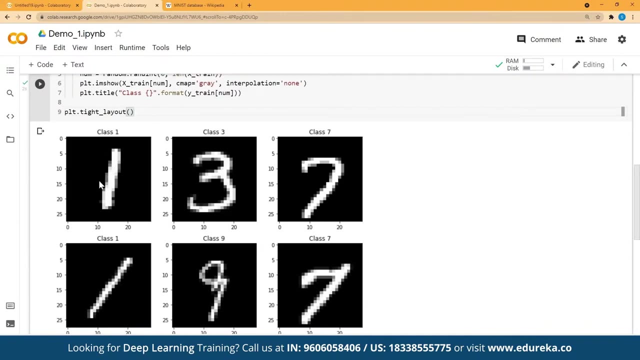 on that image. so first we are going to train that image, and once that image, once that neural network has been trained, we are going to test it. okay, so just to give you an example, how. what are the training images? these are the training images. so here, if you see there are various, this is one, this. 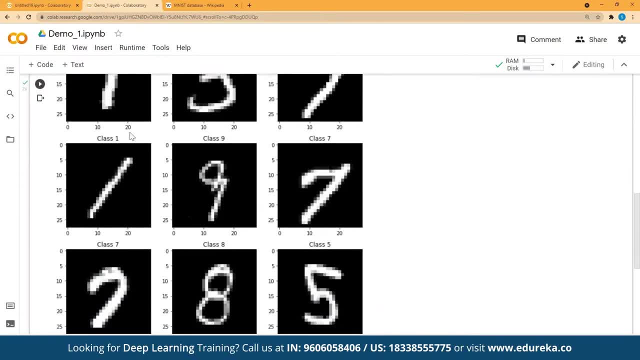 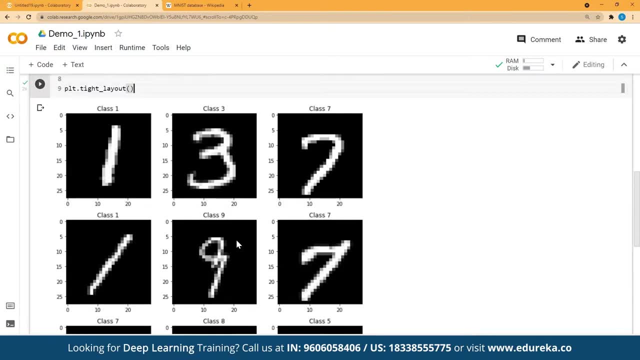 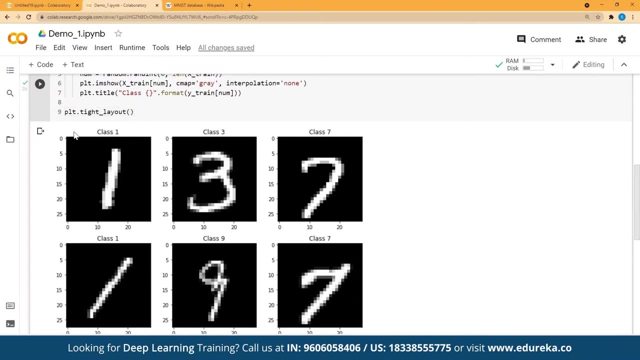 is three, this is seven, right? so these images we are going to send in an artificial neural network, as i just explained to you, and that weights will get locked and later, when we send an unknown image to it, it will identify. okay, this number represents three. okay, so this is the practical aspect of 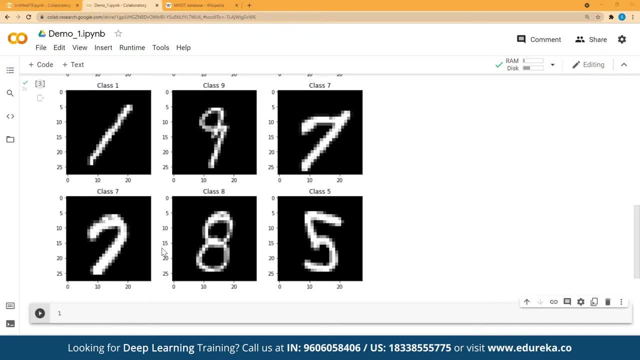 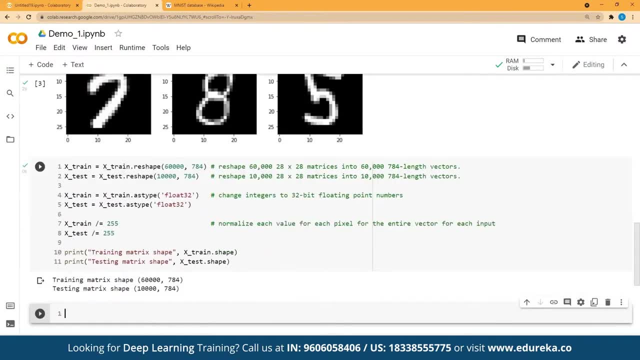 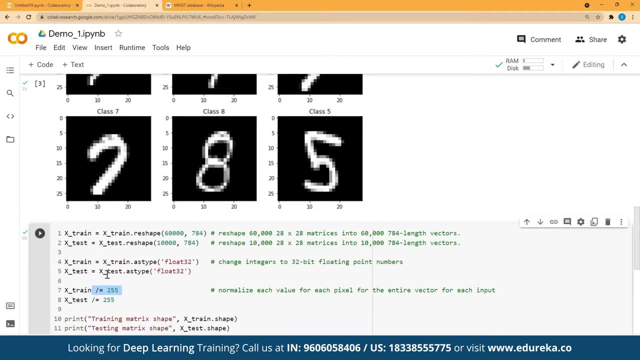 this hands-on session. okay, so i will do some data processing first of all. what i will do? i will try to scale the data here. so see, you also have to learn a few more concepts here: what is the image, what is a pixel, etc. so, if you know about that, what we are doing is dividing. 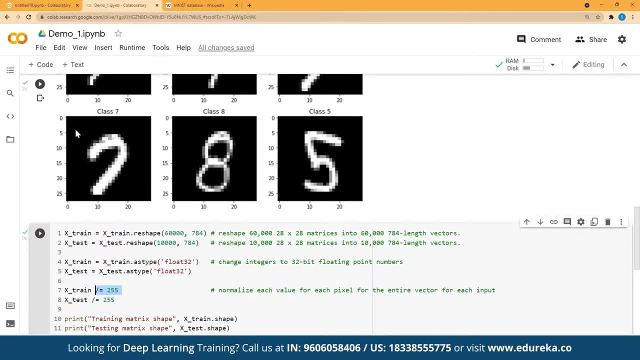 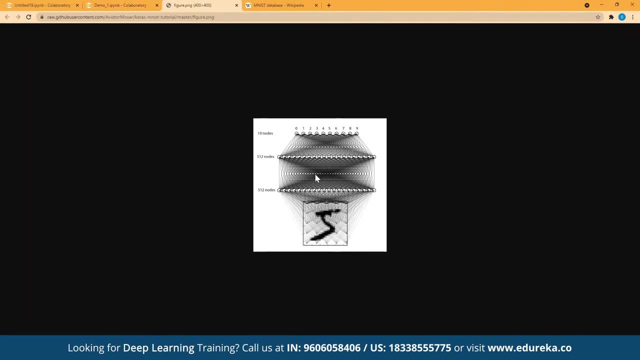 this by 255. now, 255 is the biggest pixel we can have in this. okay, so we are normalizing all the pixel values on these images by dividing it by 255. okay, now, what i'm going to train is this. what i'm going to create now is this data, so i'm going to create. 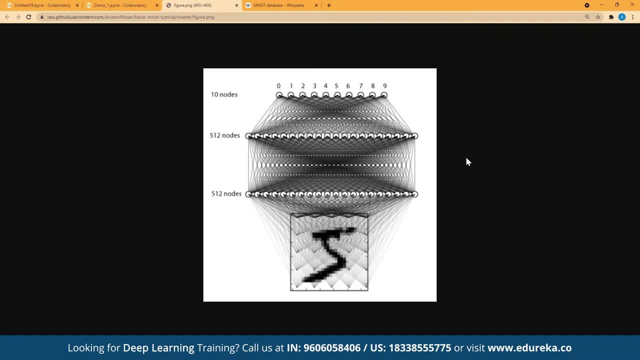 hidden layers of 512 nodes, so 512 neurons. the image will go as a input to this: two layers of 512 nodes and it will give you output of 10 variables. so it will give you the probability of what is there on this image. okay, so first of all we will train this and then we will use this. 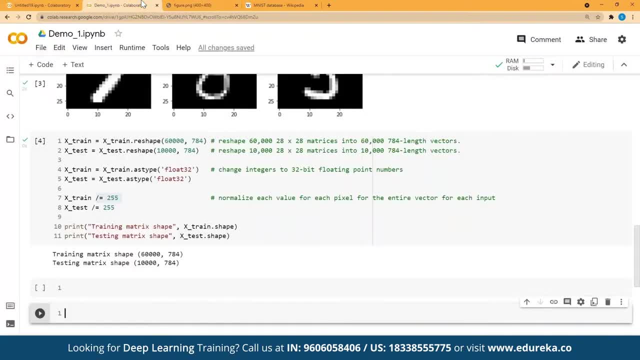 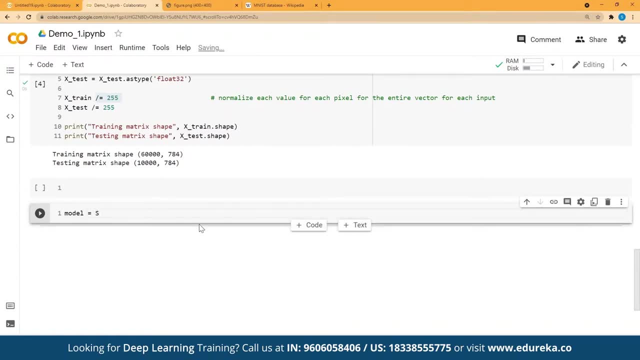 neural network, in order to get it, in order to use it. so first we are going to train it. for that i am going to create a model, model equal to sequential. so this is the code used to create a neural network. now you will see, with the ease with which we will create the image, uh. 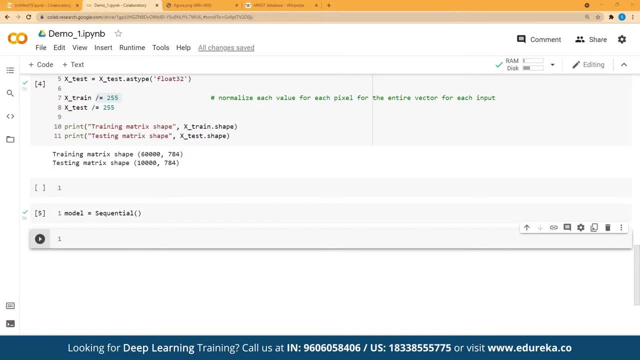 the neural network. okay, so i just need to say: please add a dense neural network. we also call this dense neural network, the image i show you. so i am telling you: please add 500, one layer of 512 neurons. so it is doing that 512 neurons. what will be the input to it? 784.. now, 784 are the number of. 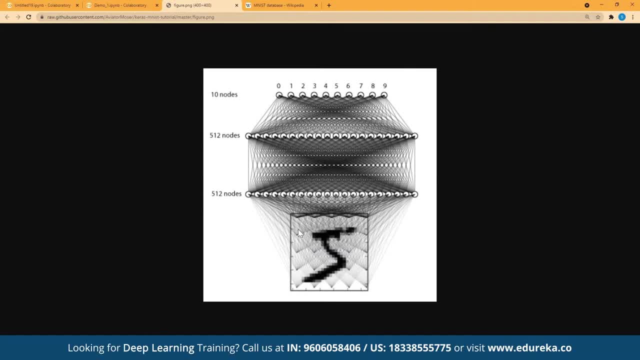 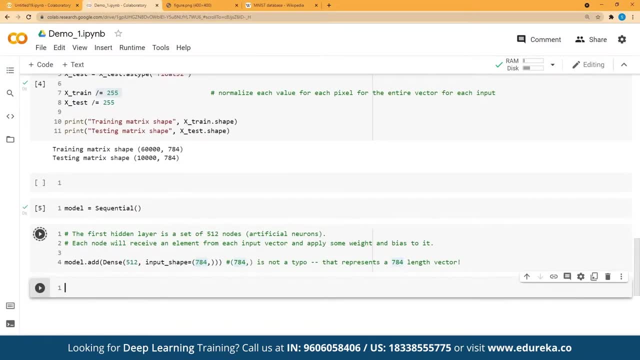 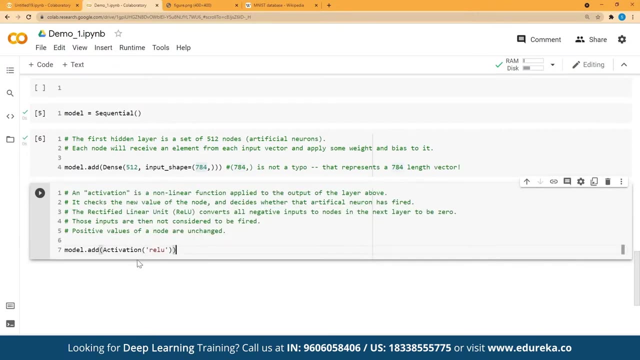 pixel values in this image, 5.. so we are telling: please take this as an input into 512 nodes. okay, so this is my first layer, first hidden layer. then what i will do: i will add a activation function. you remember i explained your activation function, so we are going to use the activation function. 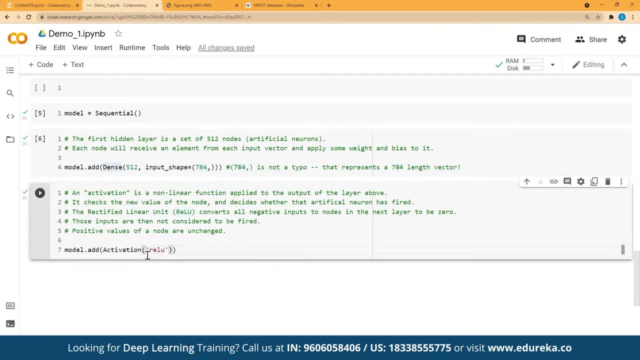 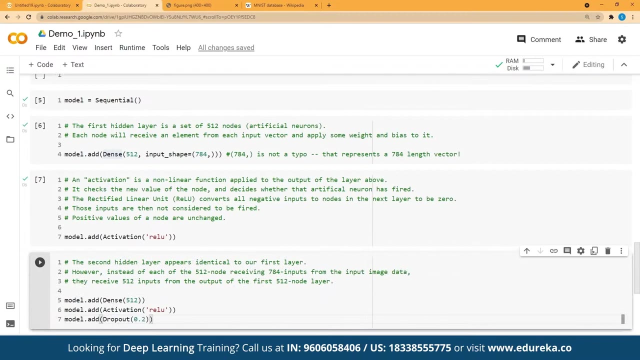 so after it goes into the dense node, we apply activation function. then again what we will have: another dense node, we will add another dense node, then we will add another activation function, then an output. so this is how we will do that. okay, now there are some concepts of dropout etc. i'll 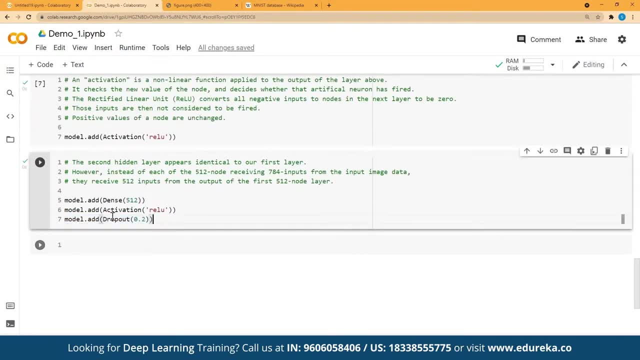 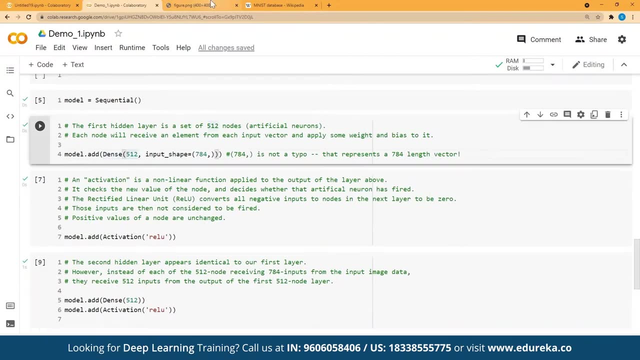 not go into those details, but those are higher concepts. here i may remove these dropout players. so for now, what i have done, i have, if you can understand, i have created the first layer. i have applied the relu function over it. now, whatever output is going, it will go to the next layer of. 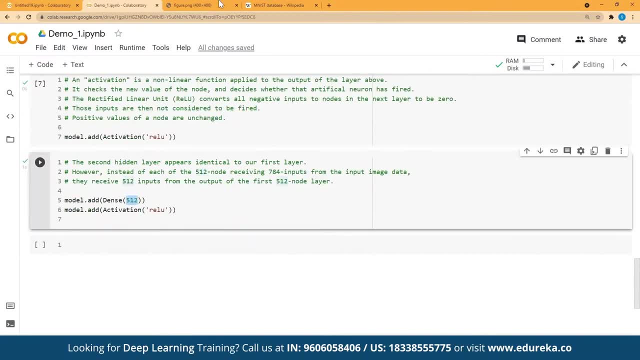 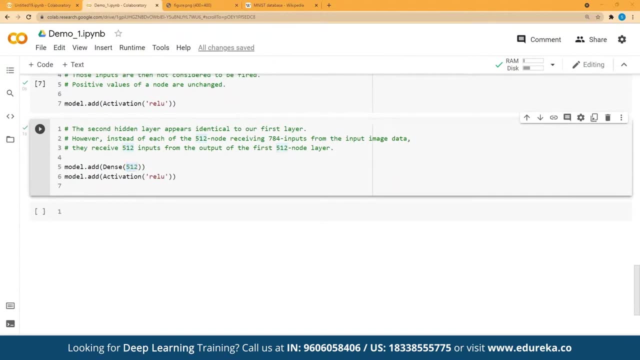 512 nodes. you can check here next layer of 512 nodes and then we will have a output layer. so now i will create the output layer. how i will create it? i will just write model dot. add dot, dense 10.. so now with this, four file. 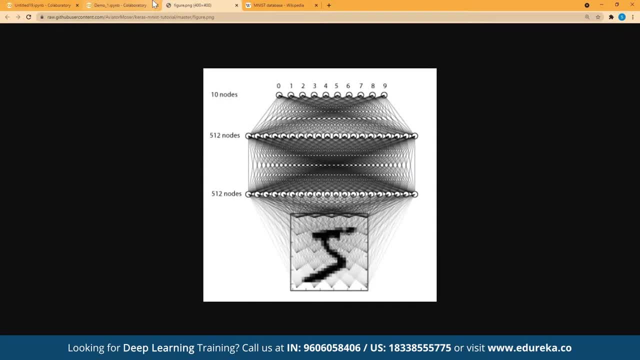 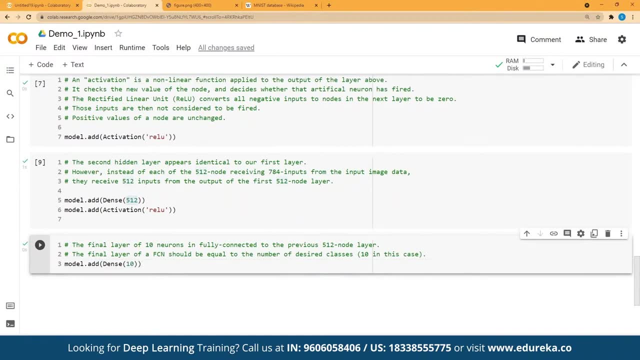 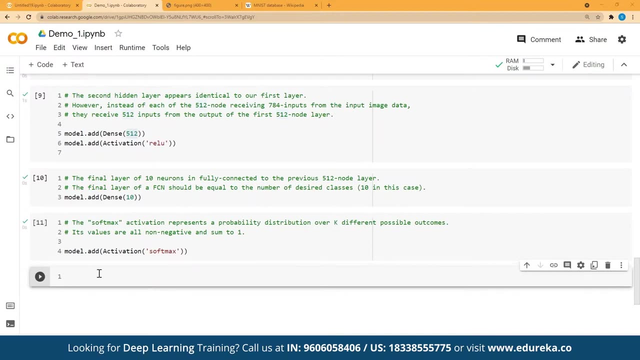 lines of code. you have created this complex neural network. okay, you have created this complex neural network. after the end layer of tens, we are going to again apply a activation function, softmax. okay, and if you want to understand the model you have developed, you can use modelsummary. it will. 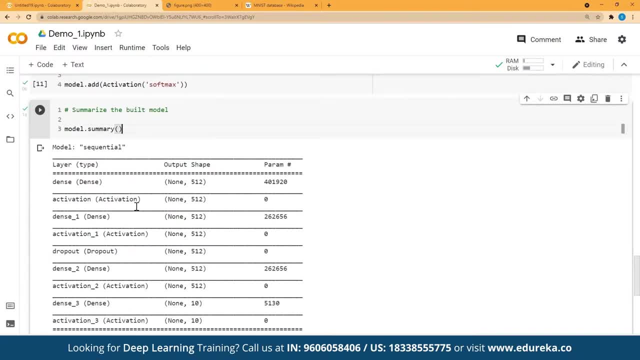 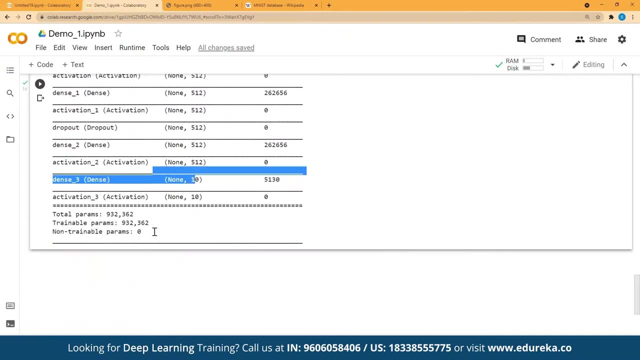 give you what kind of model you have developed. okay, what kind of model you have developed? okay. so, if you see, this is two dense layers, one and 512, and then we have created a dense layer of 10, output of 10. okay, so we create this and now what we will do, we will compile the model. 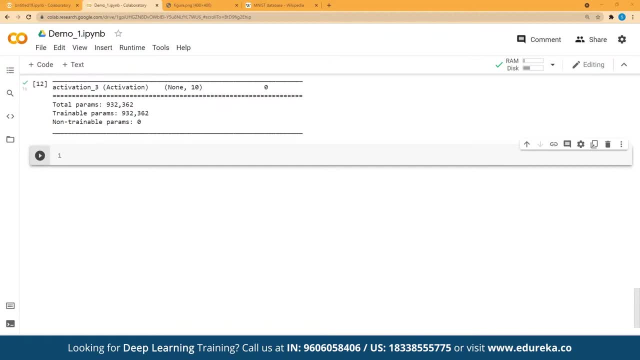 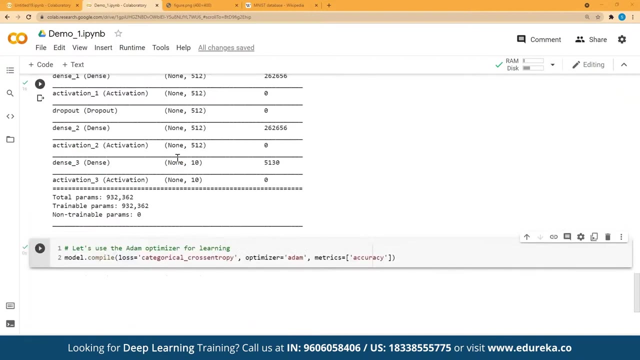 now, in order to compile it, we need to give some parameters to it. okay, we need to give some important parameters like: what is the loss function, what is the optimizer using, what is the matrix used, needs to be given to the machine, to the neural network. now what i will do once your model has. 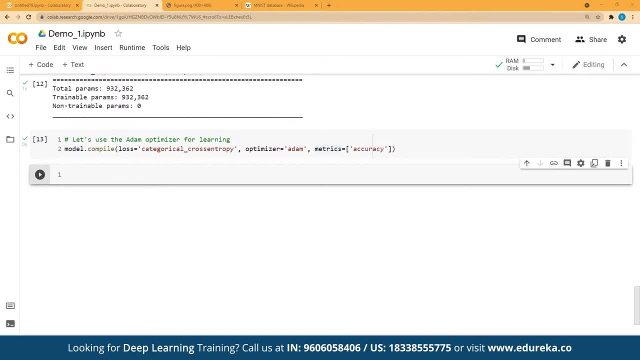 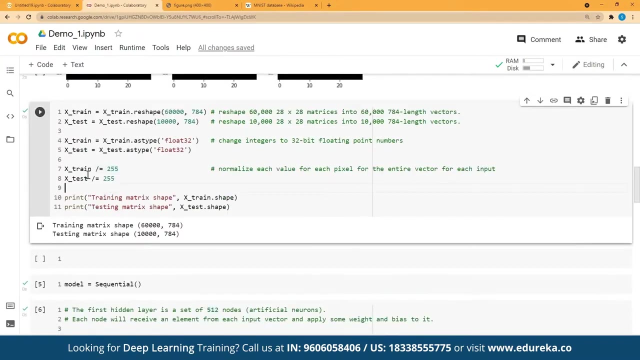 been compiled. what we will do? we will train the model. so let us train the model. and for training also, we need to pass a few parameters to it, like batch size, epoch, etc. it is staying while white grain is not defined. let me check, yeah, why train is not defined? so we have not given what is y train. 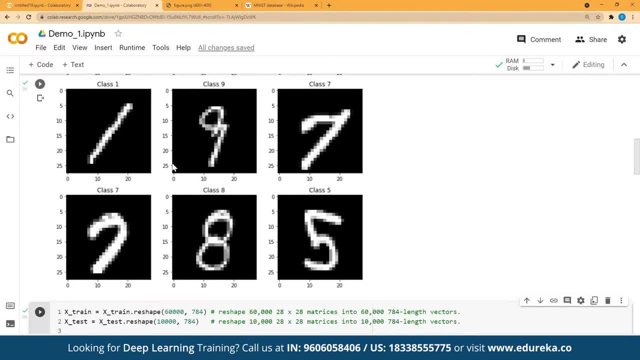 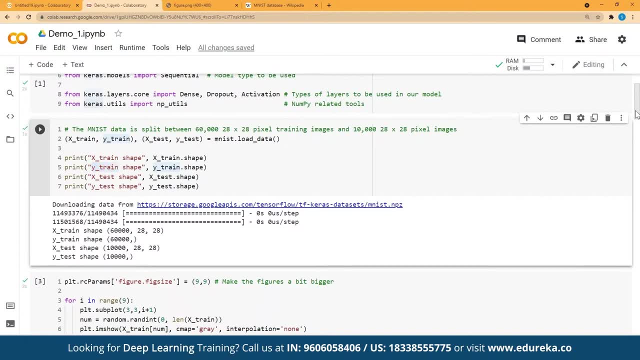 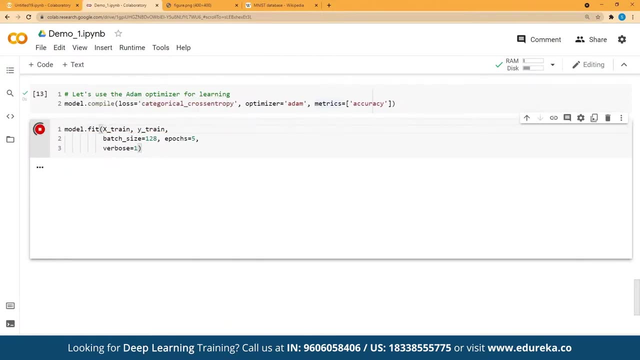 we need to dip, we need to identify that also. okay, it is small y train. if you see, we have defined y train but we have defined small, small letters y. but here what we have given, we have given capital letters y, so we will reduce it to small and run it again. okay, it is giving us an error. let me just check it. 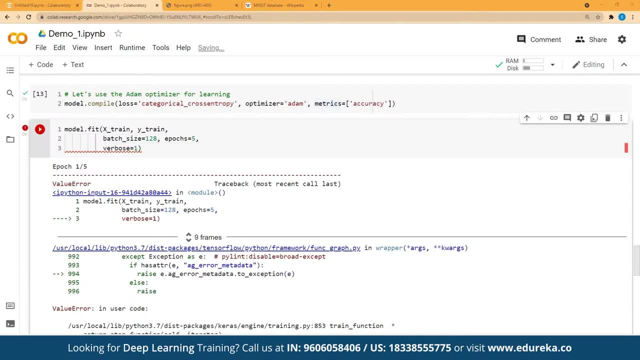 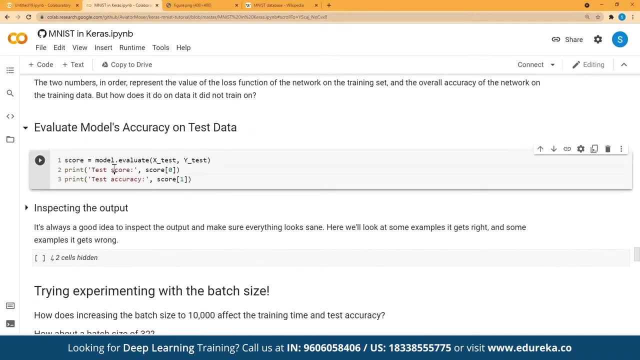 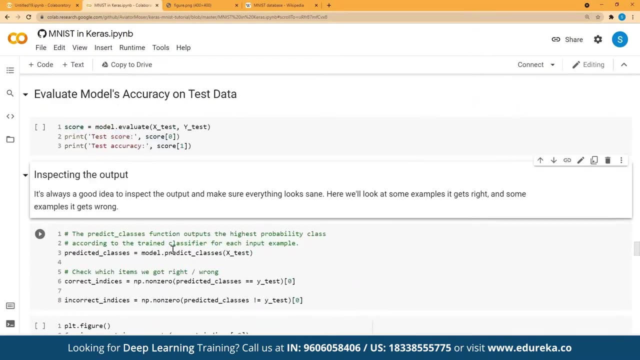 okay, okay. so it seems like there was an issue in the syntax so it was not giving a a proper result. so again, i have run it. if you see, now, once i run this model okay, and i check what is the accuracy of this model, it will give me the accuracy of that model. 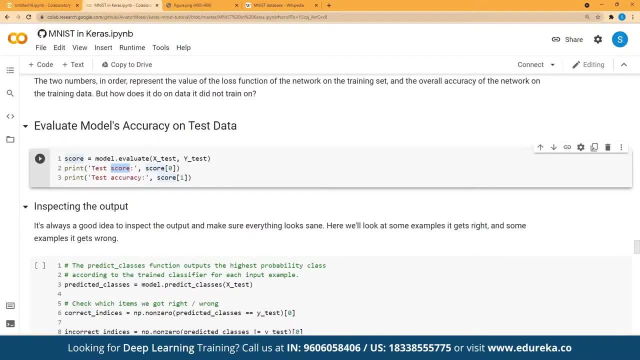 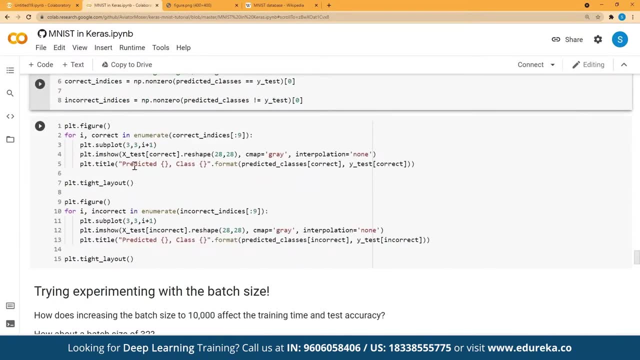 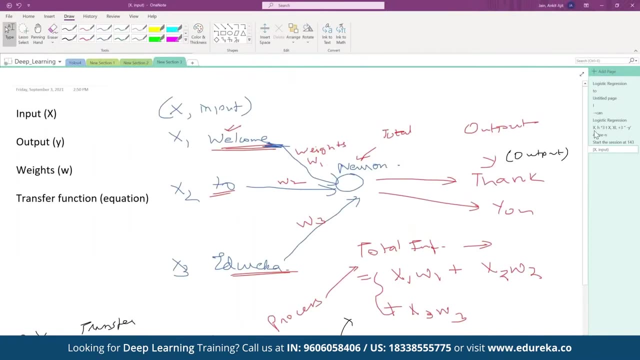 and once this model has been trained right, we can use it to predict, with some unknown data, that whether it is able to predict it correctly or not. in case it is not able to predict it correctly, okay, okay, okay, what we will do is we will change the number of neurons here, in case your model 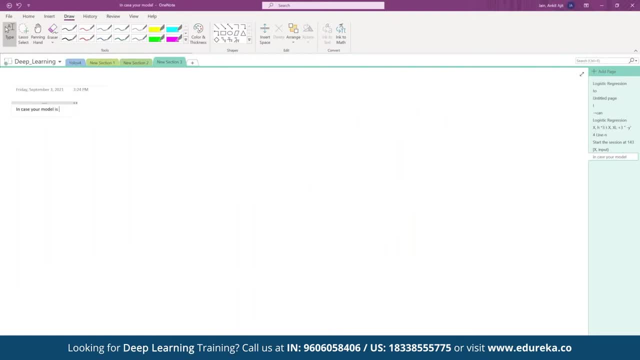 in case your model is not able to train correctly, we will change the number of neurons, the activation function, the number of layers, right? so all these things you will have to play around so that your model is trained perfectly and it is giving. it is giving proper output. what do you mean by proper output? it means that it is able to identify the 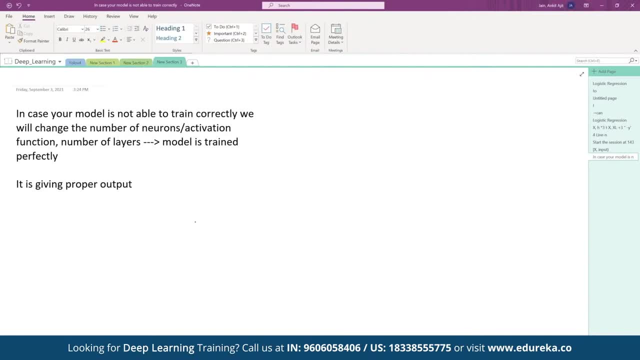 imitatrix and it is able to identify the neurons- and this part is the function of the motor- correctly? so suppose you give a input of 5, okay, suppose your image is 5, okay, and now you are giving this to your trained neural network. trained neural network. 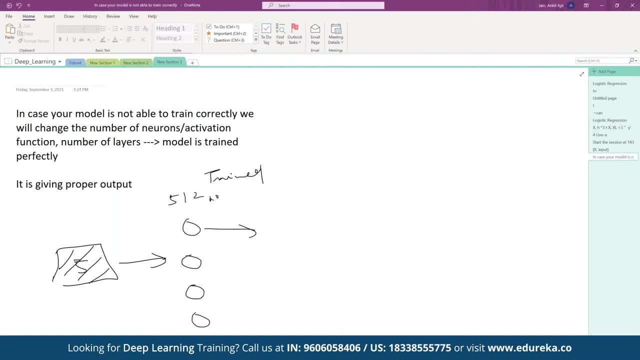 just imagine this as 512 nodes. this goes to another layer of 512 nodes and what it will predict one of the 10 numbers here, right from 0 to 9. suppose it predicts 5, then your model is well trained, but if it predicts 4, then your. 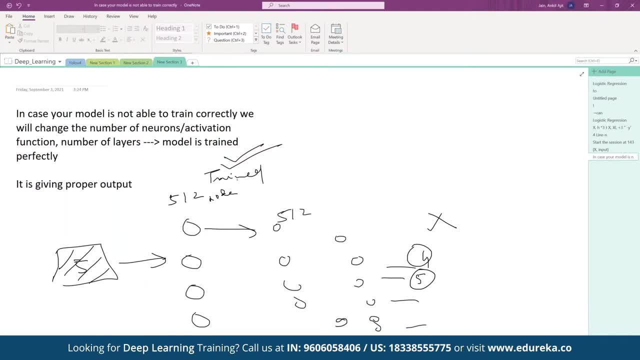 model is not trained. okay, then we will change the number of neurons, number of activation functions, number of layers, etc. in order to get more accurate results. okay, so this is how you will have to train your work neurons, and then you will be able to use your neural network, and then you will be able to 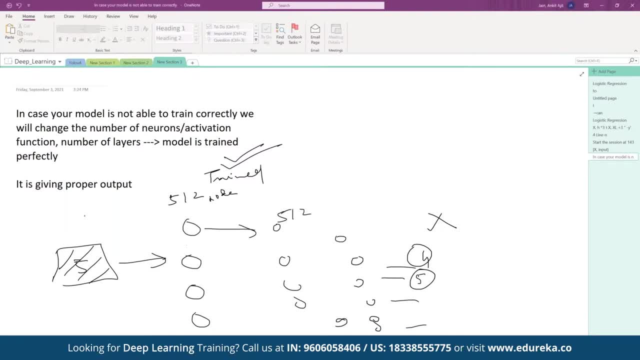 use them now. I know many of you may be having a lot of doubts here with respect to how do you decide 784 as your input? how do you set 512 as your hidden layer, right? so all this will require more deeper understanding of neural networks in terms of advanced neural network concepts, so you will have to